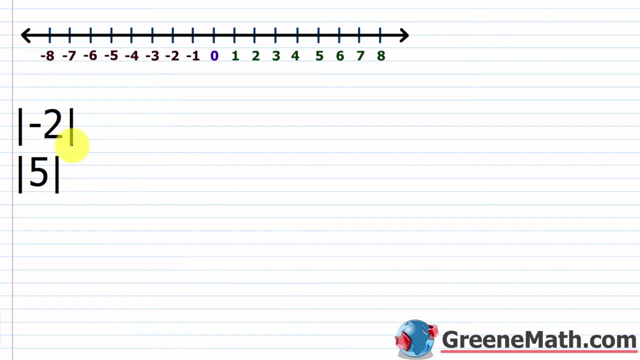 of these vertical bars. that means we want to find the absolute value of it. So the absolute value of the number negative 2 is just 2.. And so we know that from the number line we can see that negative 2 is here and zero is here, And so what I can do is I can count how far away negative 2 is. 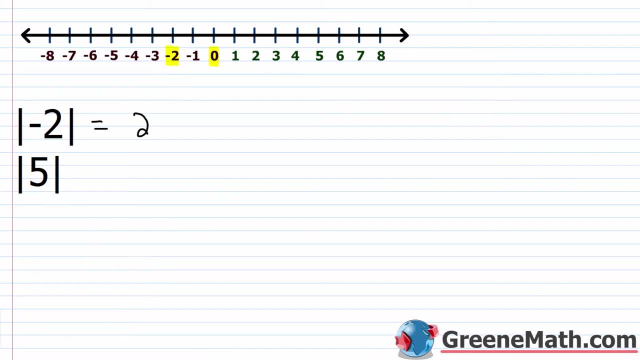 from zero. It doesn't matter the direction I move, it's just how many units I'm going to move. So we would travel one, two units to get from negative 2 to zero. So my absolute value is 2.. And we all know at this point that if you take the absolute value of a positive number, it's 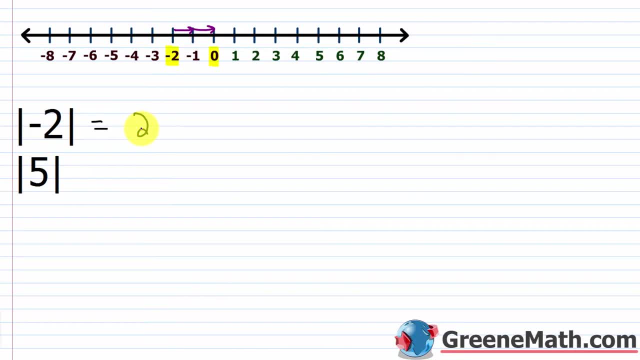 that number. If you take the absolute value of a negative number, you just make it positive. So here I took the absolute value of negative 2, just made it positive. So for the absolute value of 5, I just keep the number right, it's just 5.. And again you can demonstrate this on the number line. 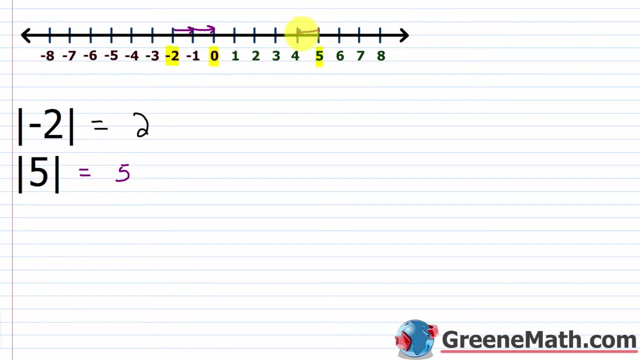 Here's 5 and again here's zero. And I would go 1, 2, 3, 4, 5 units to get to zero. And again, it doesn't matter which direction I go, we're just counting distance. It's just the same thing as. 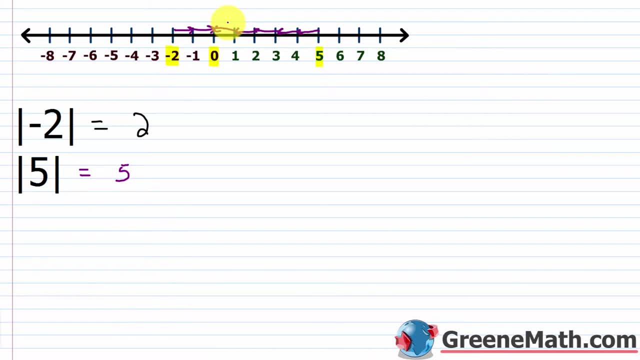 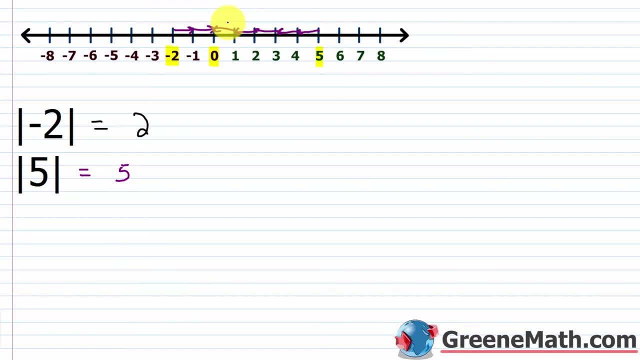 50 miles away, It would still tell me I'm 50 miles away. It wouldn't say it's negative 50 miles now or it wouldn't change based on the direction I'm coming from. 50 miles is 50 miles, Doesn't matter. 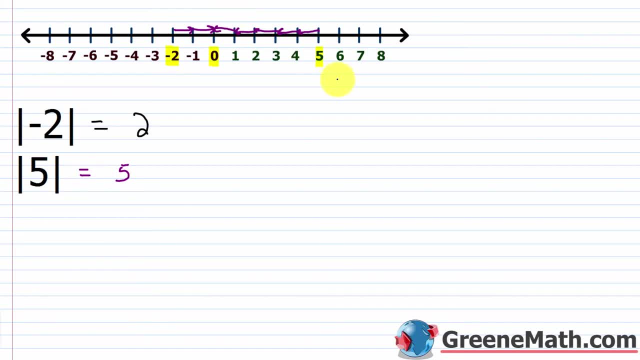 which way I'm coming from. So it's the same concept here. So absolute value can never be negative. It's a distance, So it's got to be zero or positive. And I think about this with driving again. If I tell you we've got to drive somewhere today, we can either say, nah, I don't feel like. 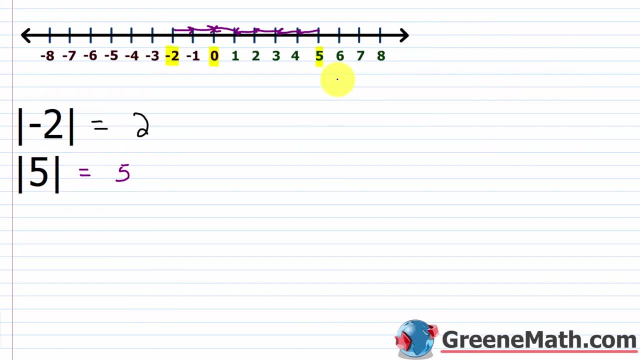 going and we drive zero miles, or we can drive some positive amount, But we can't not go somewhere or drive backwards or something silly like that and come up with a negative distance. It just doesn't work that way. All right, so now that we understand the concept of absolute value, let's look at a very 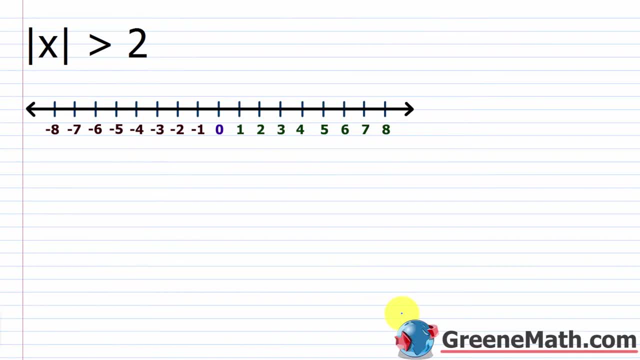 simple problem, All right, so let's take a look at the concept of absolute value. Let's look at the concept of absolute value. Let's take a look at our first sample problem. This is a very easy one that you'd see at the very beginning of the section, And it's just to understand what's going. 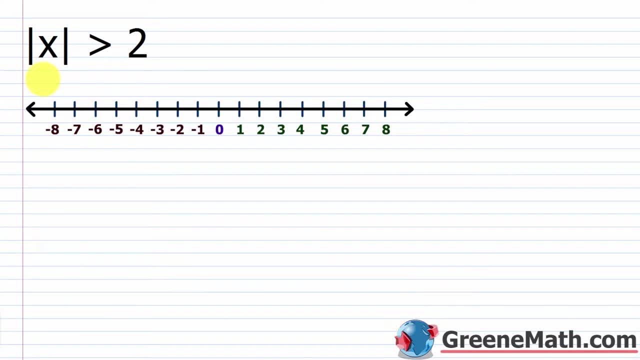 on when we're asking these questions. So the absolute value of x is greater than 2.. What are we asking for? You might want to pause the video and just think about that for a second. What are we asking for? Well, we're asking for values whose absolute value is greater than 2.. Or, if I started, 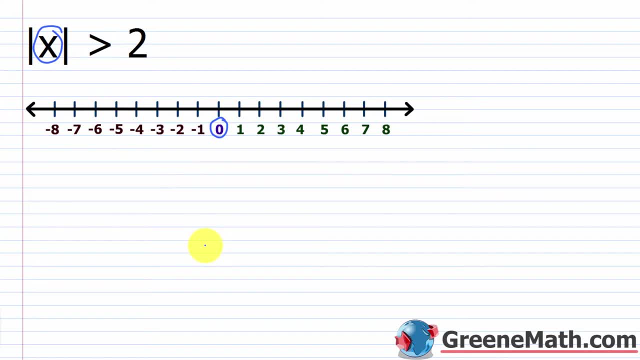 out with a hypothesis. Well, absolute values are more than 2 units away from zero on the number line. Well, if I just go 1- 2 in this direction, I know that anything larger than 2 would work. So I'd shade everything to the right here. And if I 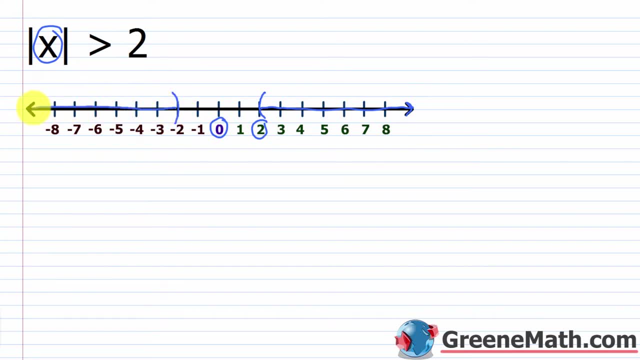 go 1, 2 units to the left. I know anything less than negative 2 would work, So I'd shade everything to the left here. So that gives me two solution sets: One where it's negative infinity Up to be, but not including negative 2. 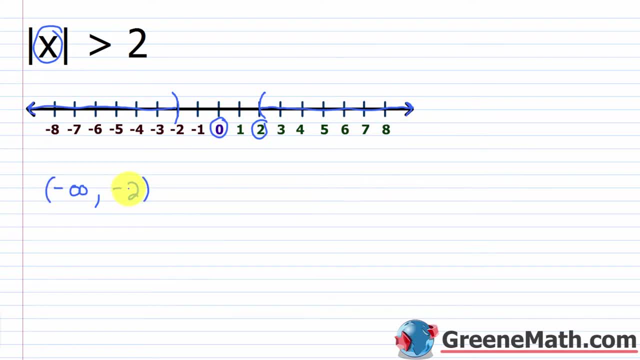 Okay, so let me start the next question. So the answer to this question is: is a solution set 2- and it's the union of this with this other guy- anything larger than 2.. So, thinking about this, any number that's involved in either solution set here would satisfy this inequality. Just pick a. 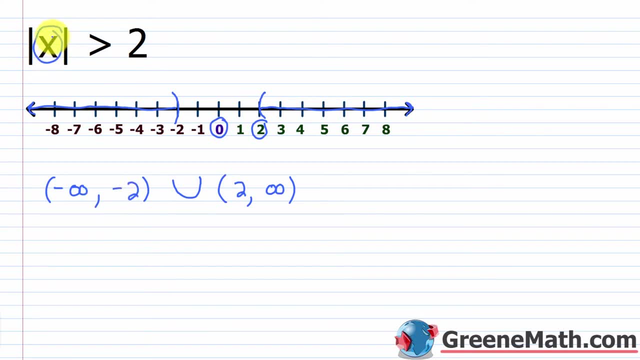 number. Let's say we pick negative 8.. Plug in a negative 8 there, take the absolute value, you get 8.. 8 is larger than 2.. Let's say you pick 3 over here. Take the absolute value of 3, you get 3.. 3. 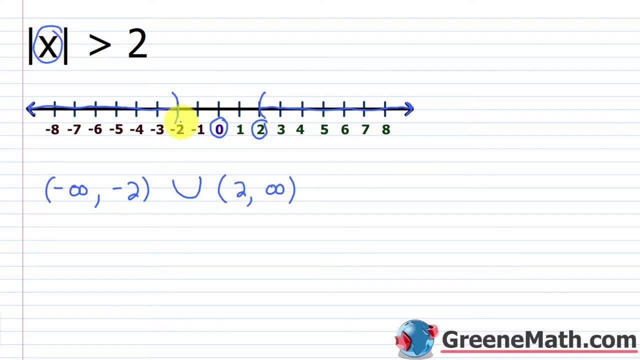 is larger than 2.. The only numbers that won't work are from negative 2 to 2, including both. If I plugged in a negative 2 there, the absolute value of negative 2 is 2.. 2 is not greater than 2.. That's false. So we know that this wouldn't work and this wouldn't work and anything in between. 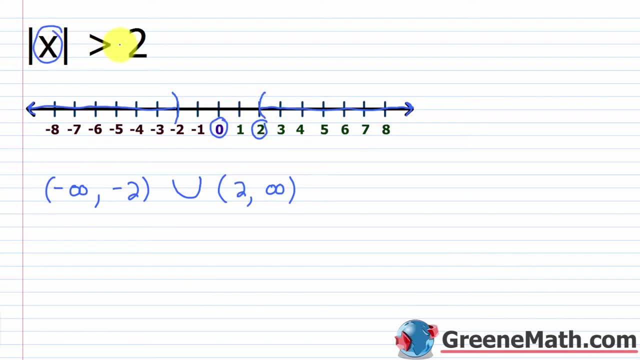 wouldn't work If I chose 1. the absolute value of 1 is 1.. 1 is not greater than 2.. So for this type of problem, where we see a greater than we're going to end up with whatever's inside the absolute, 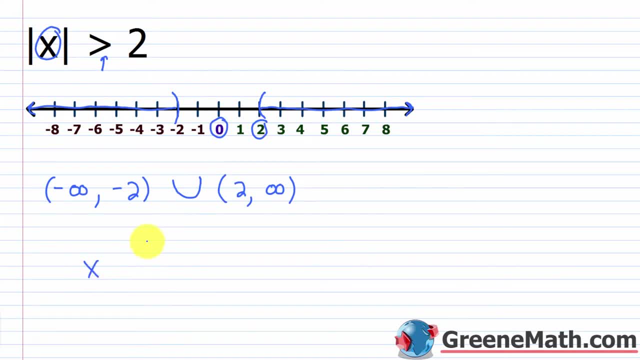 value. So in this case it's x and it's going to be greater than 2.. So in the first situation you would just remove the absolute value of r's. That's your scenario. x is greater than 2. Then you're going to have an or, So it's going to be a compound inequality. and in the second situation, 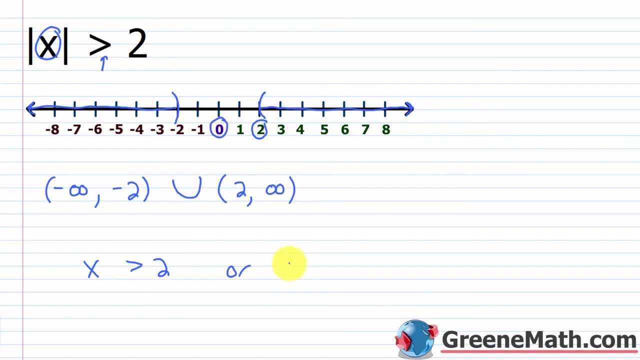 you're going to flip the direction of the inequality, So I would have x. I'm going to flip this and I'm going to make this part right here, whatever's on the right side- negative. Now you might say: where does this go? I'm going to make this part right here negative, So I'm going to. 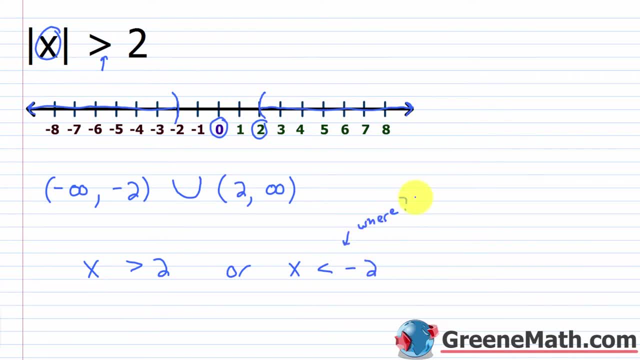 here is going to have x come from. where does this come from? That's a common question you get in class because this one right here. this is very straightforward. everybody understands that x can be greater than 2.. That makes sense. But for x to be less than negative 2, yeah you can see it here. Once you kind of think about it, it makes sense. But once you get to the next example it's like where did that come from? 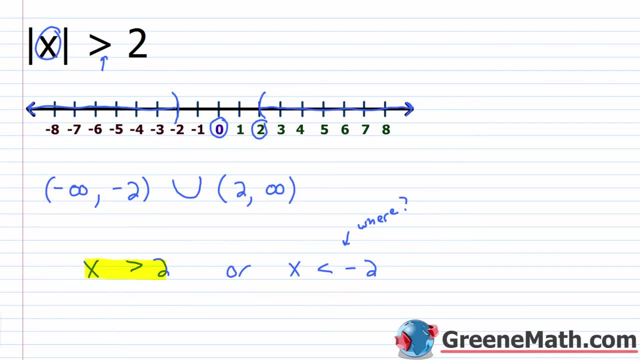 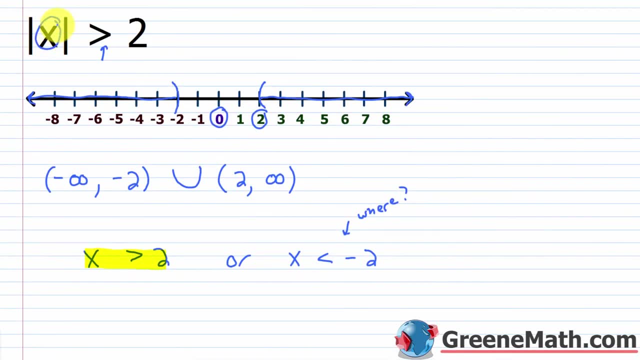 come from. Well, all you'd have to do is think about absolute value for a second. If x, let me kind of scroll down a little bit. Remember, I'm plugging something into the absolute value operation. I can think about negatives as well, So the negative of x, the negative of x could also. 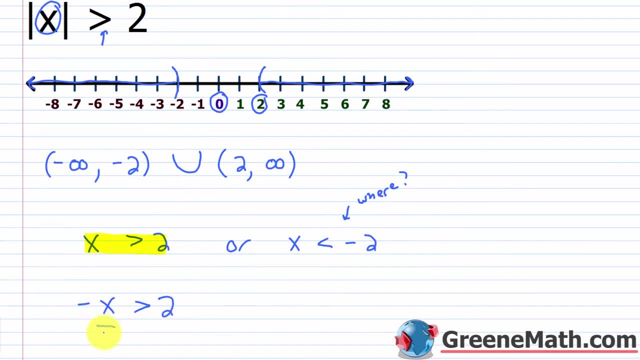 be greater than 2.. And if I divide both sides by negative 1 to get x by itself, what happens is I have to flip the direction of the inequality symbol, So this is going to become a less than right, which is what I have there. And then this divided by this is just x, And then 2 over negative. 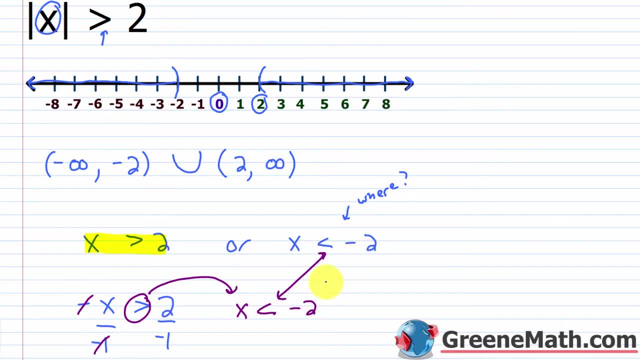 1 is negative 2.. So that's where it comes from, And once you see me do that, you can remember to do that on your own in the next example, And then you won't have to think about: well, what's the? 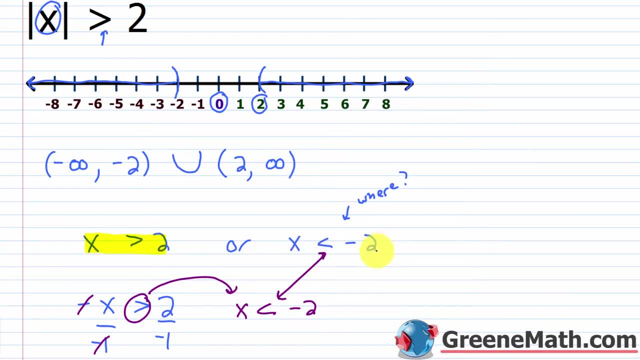 other scenario. This one's straightforward, This one everybody forgets. OK, So it's: x is greater than 2 or x is less than negative 2.. If you had a generic example like the absolute value of x is, let's say, 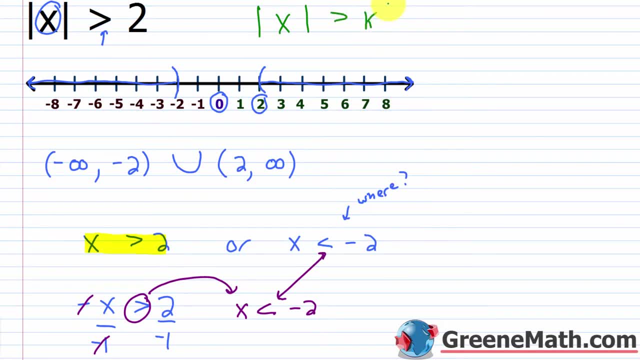 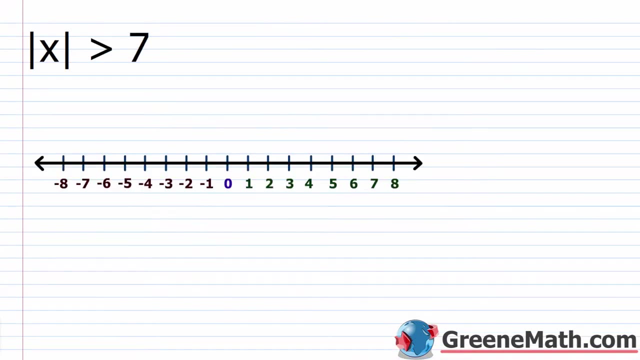 greater than I don't know. let's say some variable k. Well, this sets up to: x is greater than k, or x is less than negative k. just following this format here, In this case k is just 2, right, So x is greater than 2 or x is less than negative 2.. So here's another example. 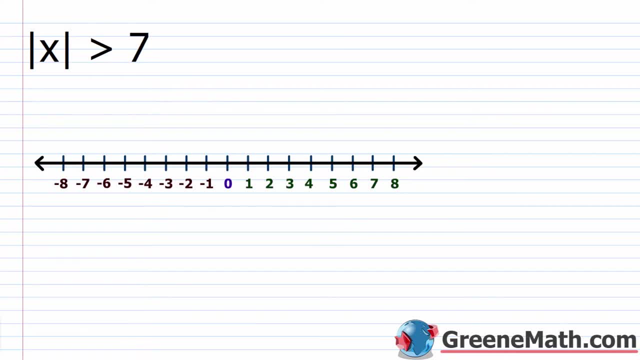 very similar We have: the absolute value of x is greater than 7.. So, again, what we're asking for here is give me numbers whose absolute value or distance from 0 is larger or greater than 7.. Well, I know, anything larger than 7 would work. 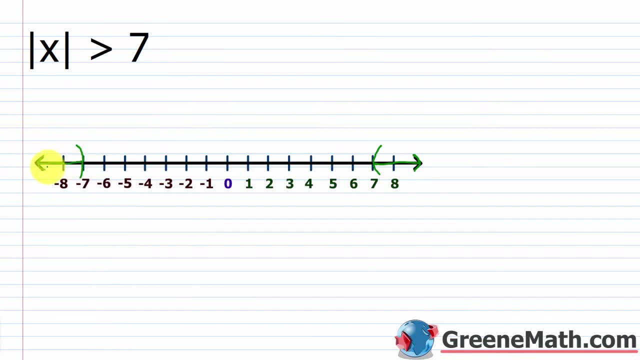 And also anything less than negative 7 would work, because if I look at 0 here, if I count 1,, 2,, 3,, 4,, 5,, 6,, 7,, yeah, anything to the left of negative 7, that works, And then again 1,, 2,, 3,. 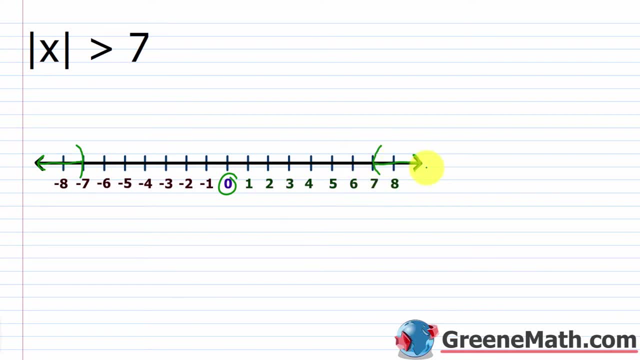 three, four, five, six, seven, Yeah, anything to the right of seven, that works as well. That's a distance that's greater than seven units from zero. But again, we don't need to pull out a number line every time. If I have a greater than remember, use your generic example: The absolute. 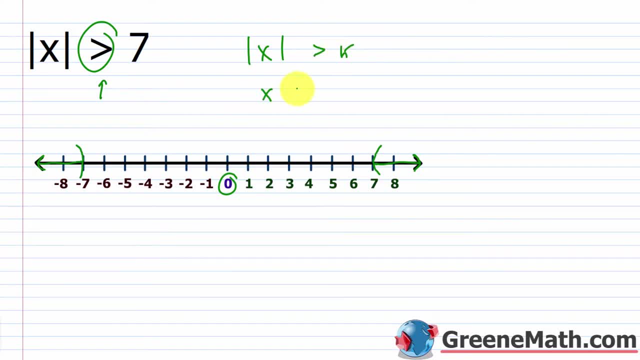 value of x is greater than k sets up to x is greater than k or x is less than negative k. So x could be greater than seven or x could be less than negative seven. And again, let's do this one more time. Where does this come from? Well, I can take this part right here and say: well, 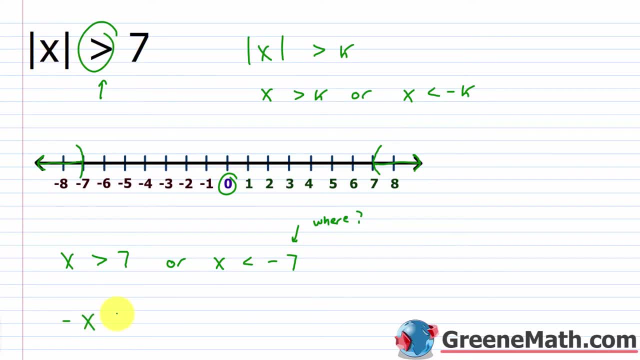 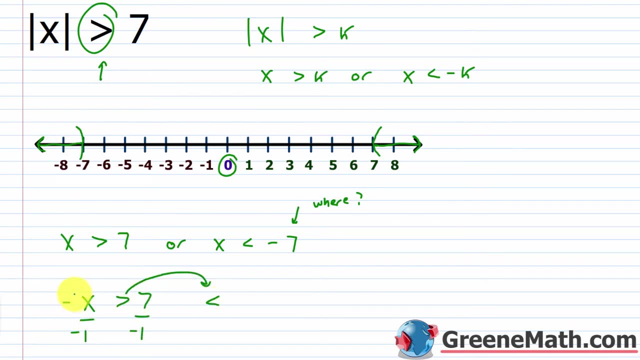 the negative of x could also be greater than seven. The negative of x could also be greater than seven. I divide both sides by negative one. This gets flipped, And so you'd have this cancels. with this, x is less than negative seven. So that's where this came from. And again, 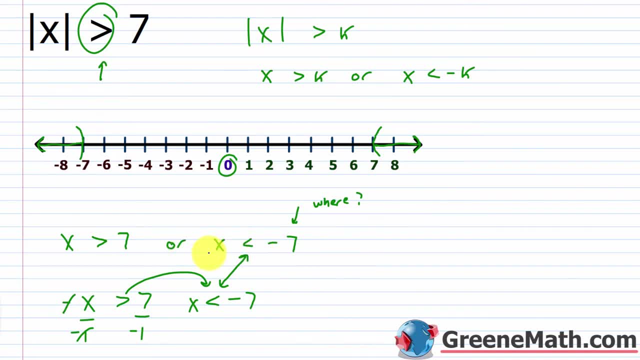 you can do this one more time. So x could be greater than seven or x could be less than three, And you might be asked to write this in interval notation And with: or it's the union of the two solution sets. So I would have from negative infinity up to, but not including, negative. 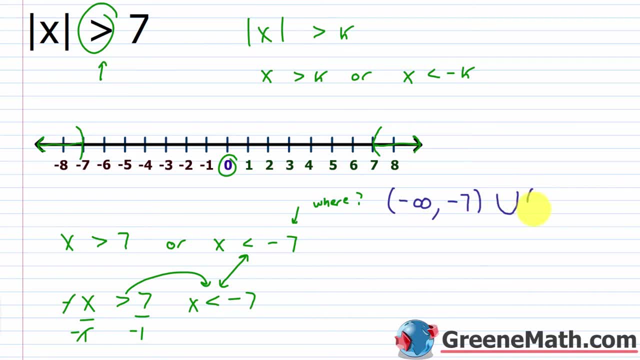 seven, And it's the union with the other solution set which is greater than seven, out to infinity. All right, so now that we've dealt with the greater than scenario, let's talk about the less than scenario. So we have the absolute value: of x is less than three. So here, 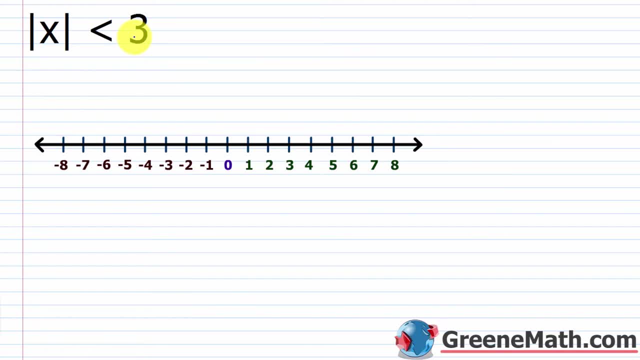 x can be any number that is less than three units away from zero, So anything less than 123 units. so it can't be three, but it can be anything less than three. So 123 can't be negative three, but it can be anything greater than that. So basically, 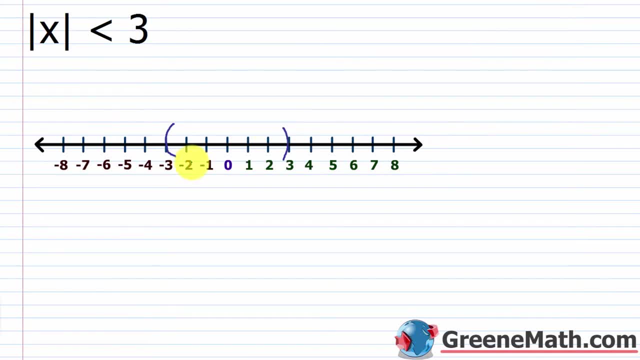 it's the numbers that are between negative three and three shown here And again. the first scenario to do this, where x is just simply less than three, it's very straightforward: just remove the absolute value bars and you have x is less than three. For the other one. 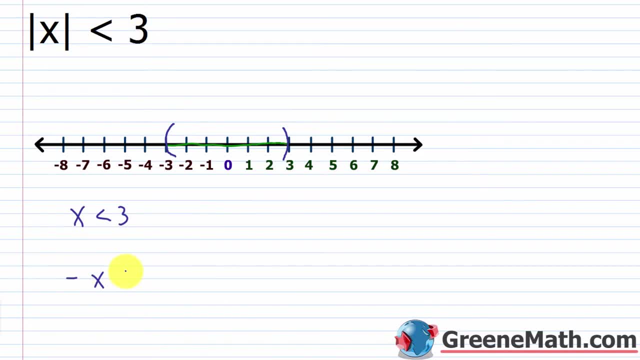 you have to think about. the negative of x is less than three. Well, if I divide both sides by negative one, what's going to happen is this gets flipped. this is now greater than this cancels with this and I'll have: x is greater than negative three. So this sets up a compound. 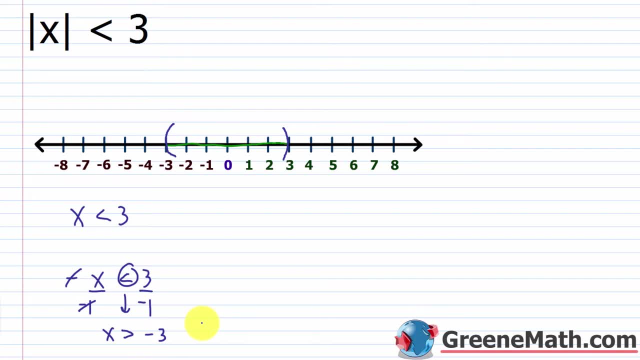 inequality with and and. really you could write this as a three part inequality where x is in the middle. So x is going to be greater than negative three and it's less than three. So it's between negative three and three. And again, I'll just kind of erase this real quick- You could write: 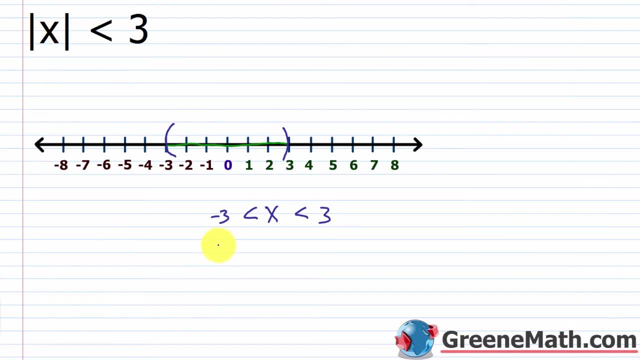 something like this: an interval notation. pretty easily, you would put negative three next to a parenthesis comma three. So that's your solution set for this. Now, generically, if I had the absolute value of x is less than k. what I want is remove the absolute value bars. you'd have x. so I want to be very shoot using straight out an partialalin, And I want to have x equal to that. Now you'll have interesting fucking idea that that would be just fine to have the type that you want to write in yourmetros, But the idea is that the one that would be the top is the bottom and my model. 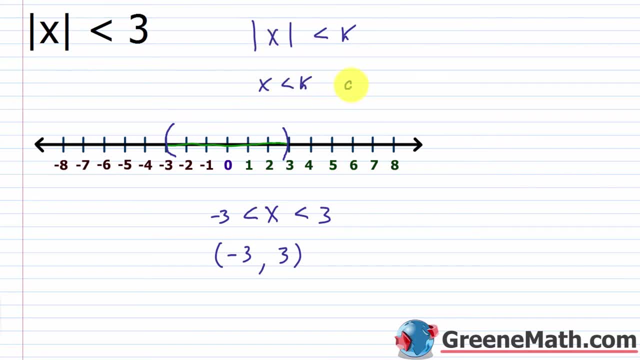 would be totally different because basically, when the curve is over the top and the other end will be higher than you, you'd have X is less than K then and you would also have remove the absolute value bars. you'd have X, flip the direction of this, you'd have greater than and make this negative, so negative. 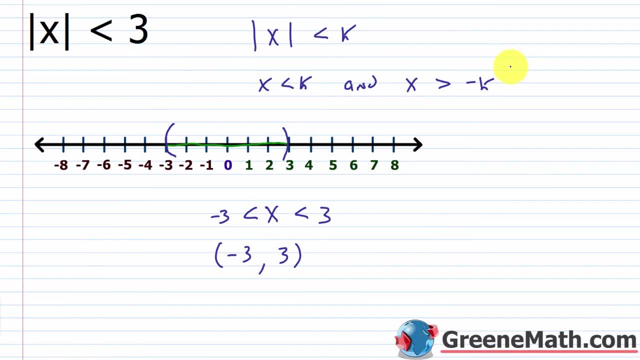 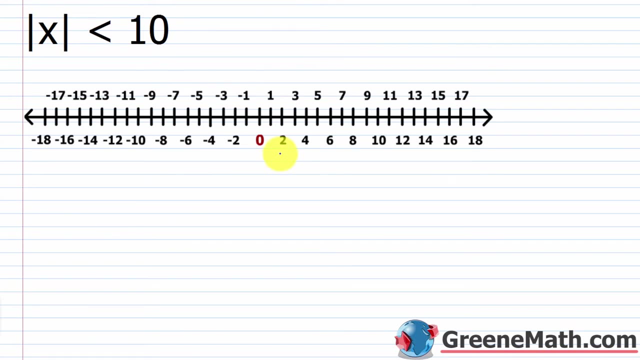 K. in each case, you basically do the same thing, but in one situation you have or, which is, when you have a greater than, and when you have a less than, you have an, and so let's take a look at the absolute value. of X is less than 10. so, following our last example, we know that X would be what it. 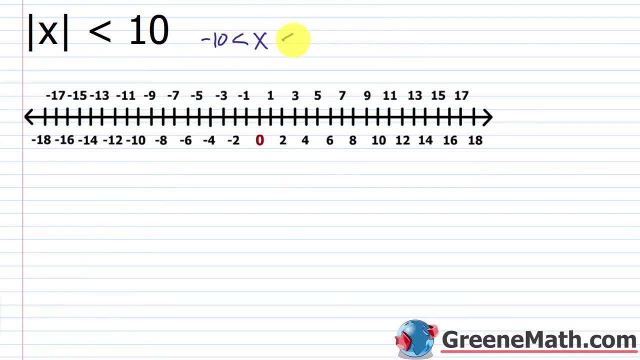 would be greater than negative 10 and less than 10. right, you see how fast I do that, so once you've got kind of the rules down, you can do these very quickly. but again, think about this as a concept. the absolute value of X is less than 10. so from 0, what's less than 10 units away while we go to. 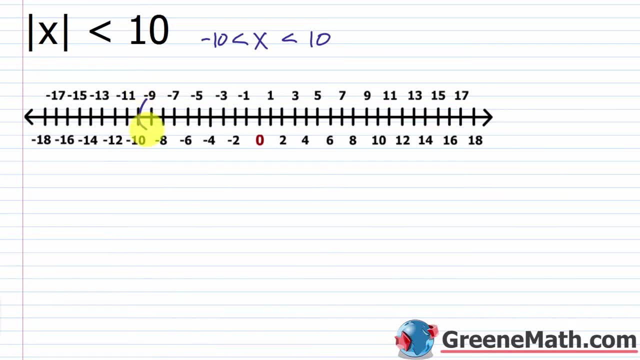 negative 10, and I would put a parenthesis facing to the right, okay, because anything that is negative 10 or further to the left wouldn't work. their absolute value or their distance from 0 is 10 units or larger. I'm looking for less than 10, so 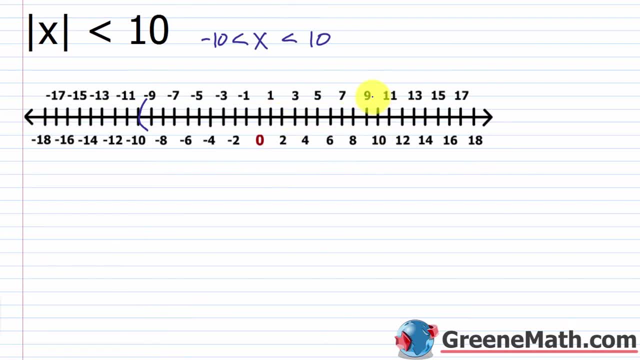 also going this direction. I would stop at 10. I'd put a princess they're facing to the left again. anything that's 10 or larger won't work, because the distance from 0 is 10 or more and we want 10 or less. so then we want all the values in both of them to be less than or equal to or equal to 0. 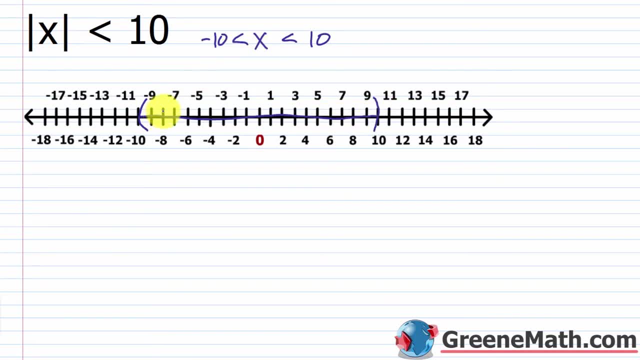 between. here again, X can be larger than negative 10 or less than 10. so an interval notation: I would just simply write a negative 10 comma 10, with a parenthesis next to each and again, just to go through this one more time. we know that X could be less than 10. the other scenario is the negative of. 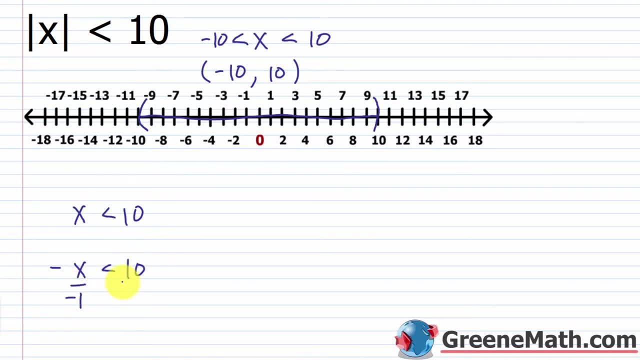 X could be less than 10. we divide both sides by negative 1, this flips and we end up with X is greater than negative 10. so this sets up the compound inequality: X is less than 10 and X is greater than negative 10, which we write as a three-part. X is greater than negative 10 and 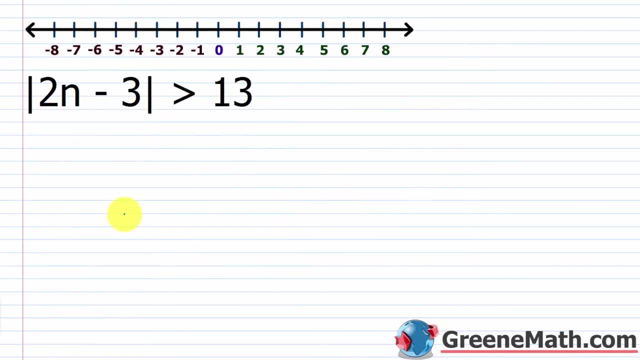 X is less than 10. okay, so that's where all this comes from. so now let's look at one that's a little bit more challenging. this is something you'll see at the very, very first part. so we have the absolute value of 2: n minus 3 is greater than 13, so the first thing to make sure of is that. 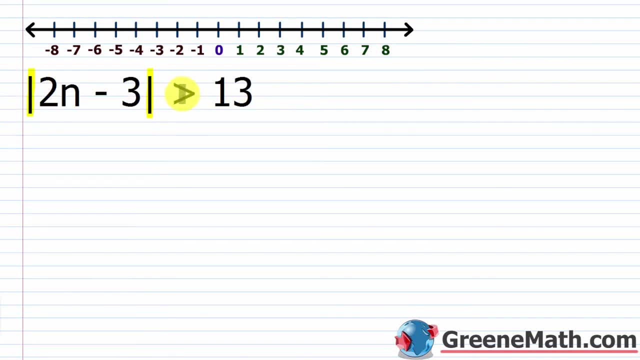 is isolated. so this is isolated. you have an inequality symbol and then some number. now the next thing you think about is: is it a greater than or is it a less than? okay, in this case, it's a greater than. so, with a greater than we have, or? all right, we set up a compound inequality with or. 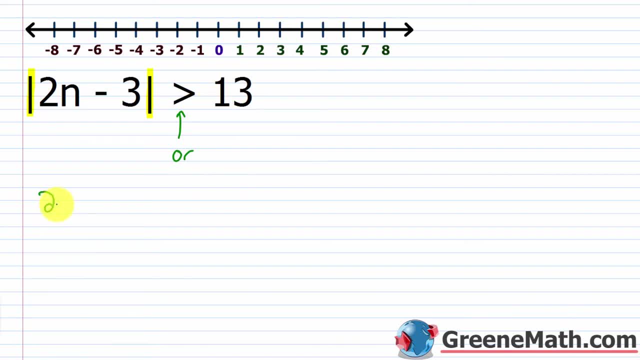 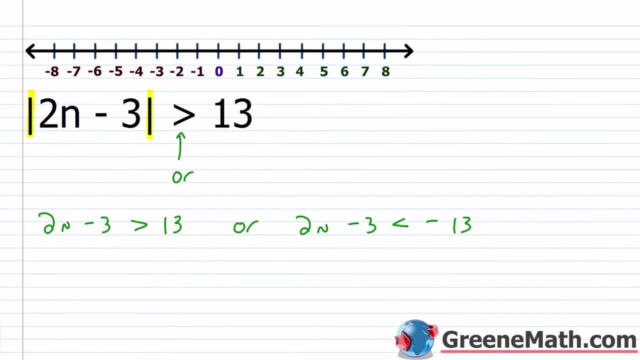 so the first one is: remove the bars, so 2n minus 3 is greater than 13 then. or the second one is: remove the bars, so 2n minus 3, flip the sign so it's a less than make this negative, so negative 13.. again the easy way to remember this. go back to your generic example: the absolute value of x. 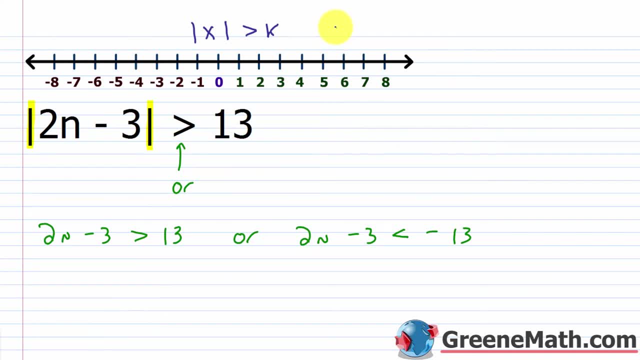 is greater than k. so this turns into x is greater than k or x is less than negative k. just use this as an example on the first few and you'll remember. the first one is: just remove the bars, as we have here. we just remove the bars we have. x is greater than k. the second one is: remove the bars. 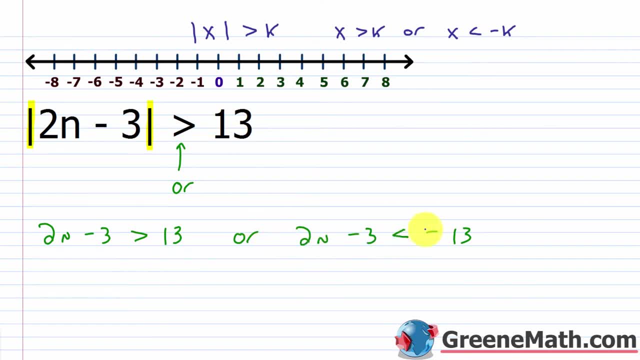 flip the sign, make it negative. so we remove the bars, we flip the sign from greater than to less than. we made 13 negative 13.. and again where this comes from, if i took the negative of this, so let's say i have the negative of this whole expression: 2n minus 3 is greater than 13. what i can do is: 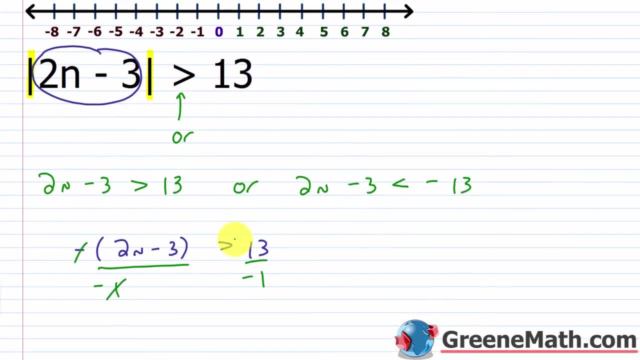 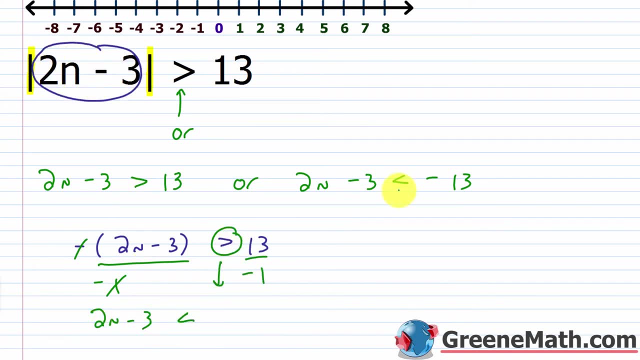 i can take the negative of this and i can cancel this, divide this by negative 1, but this gets flipped, so you get 2n minus 3, which is this flip the sign. okay, that's why we flip here, and then we make this negative, so this is negative 13.. so, again, that's where this is coming from. 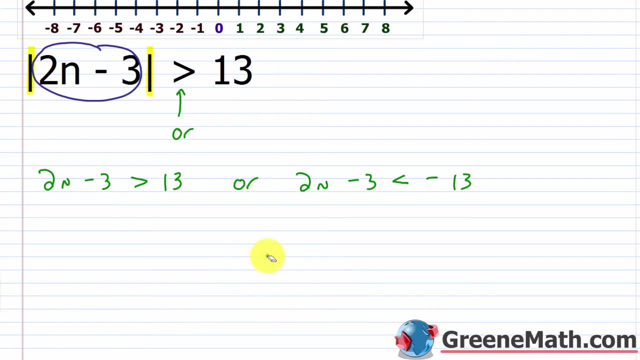 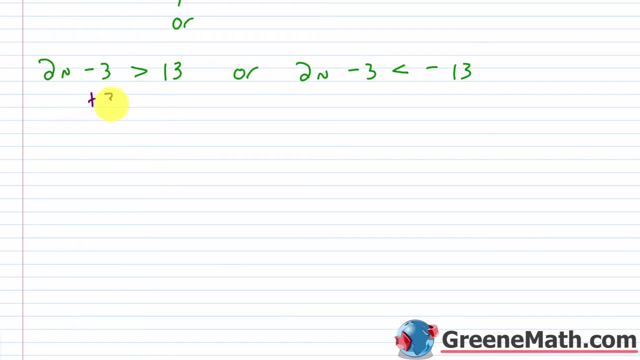 all right. so let's erase everything. let's get our solution. let's scroll down a little bit. so i just want to solve this like i normally would. so i'd add three to each side here. that will cancel. 2n is greater than 16.. divide both sides by 2 and i get n is greater than. 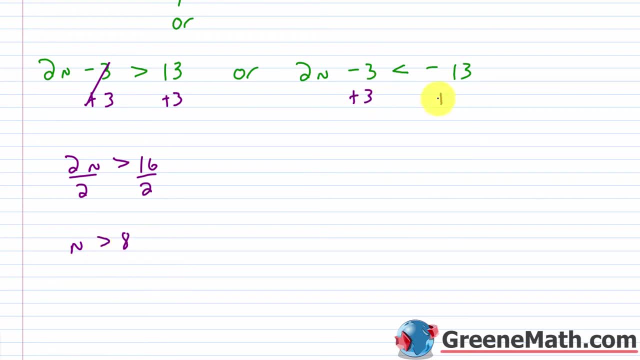 8. over here i'll add 3 to each side. that'll cancel and i'll have 2n is less than negative. 13 plus 3 is negative 10.. divide each side by 2 and we'll get that n is less than negative 5.. 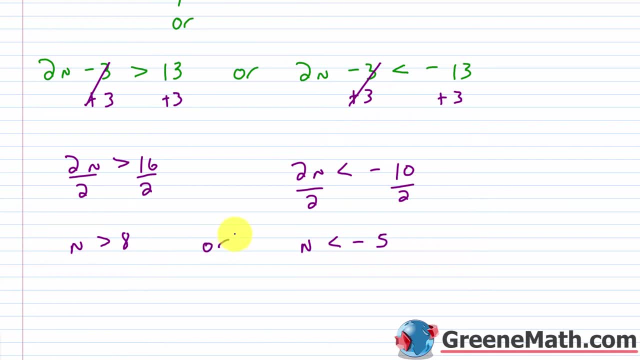 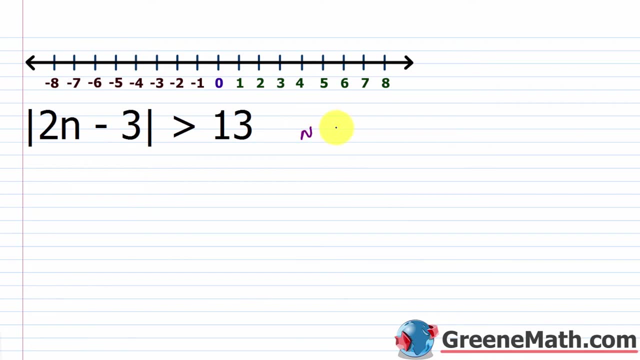 so i get n is greater than 8 or n is less than negative 5.. so let's go back up and notate this. so your solution here would be again: n is less than negative 5 or n is greater than 8.. in interval notation i could write from negative infinity: 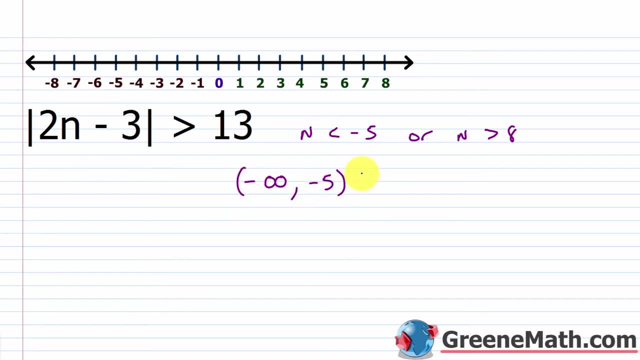 up to, but not including negative 5, and it's the union with this other set which is anything larger than 8, out to infinity. now, graphically, at negative 5, i'd put a parenthesis facing to the left and i'd shade everything this way. and at 8, i'd put a parenthesis facing to the right and i'd shade. 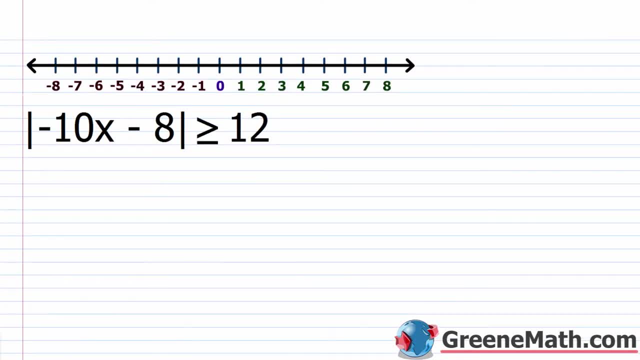 everything this way? all right, let's take a look at another one. so we have the absolute value of negative. 10x minus 8 is greater than or equal to 12.. so again i'm looking at a situation with a greater than. it doesn't matter that it's a greater than or equal to, it's just going to change the 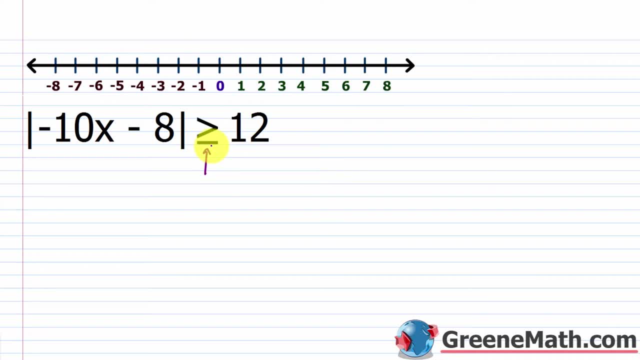 notation a little bit. if i have a greater than involved, or greater than or equal to, it's a compound inequality with or so. if i have a greater than involved, or greater than or equal to, it's a compound inequality with, or so. i remove the absolute value bars, so negative 10x minus 8 is greater than or equal to 12. 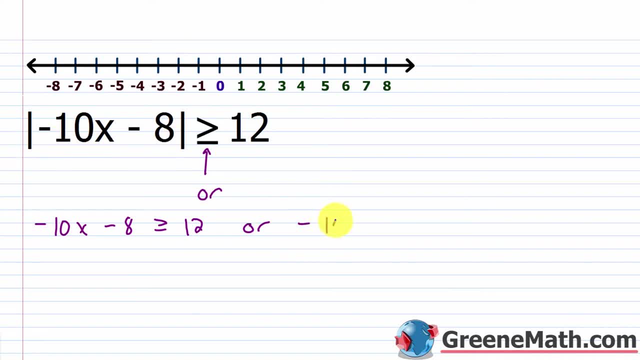 then, or remove the absolute value bars, negative 10x minus 8, flip the sign. so now this is a less than or equal, to make this negative, so negative 12.. and again, that comes from the fact that i can have the negative of this be greater than or equal to 12.. i divide both sides by negative 1. this 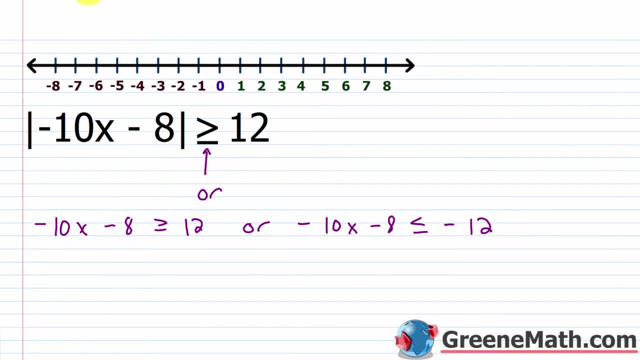 gets flipped. it's just that simple. so let's go ahead and solve each one here, so we'll have plus 8 and plus 8 that cancels negative. 10x is greater than or equal to 12, plus 8 is 20.. divide both sides. 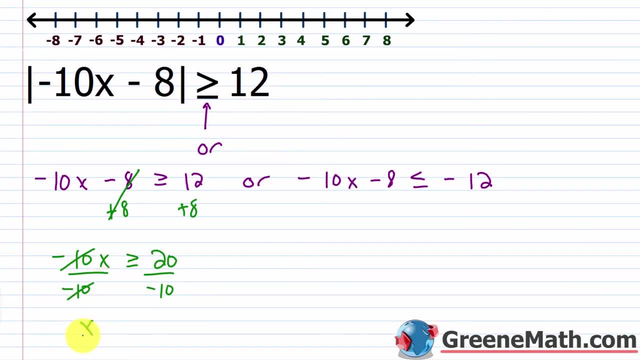 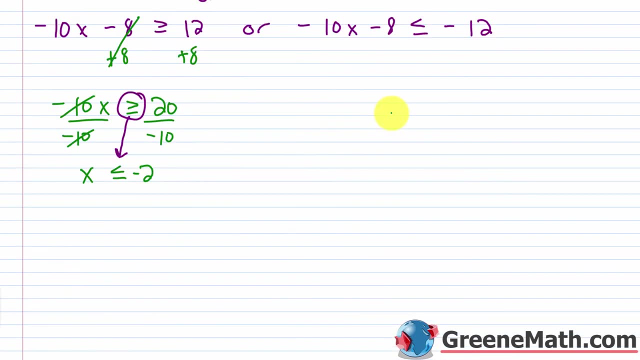 by negative 10 and this will cancel of. x is less than or equal to 20. divided by negative 10 is negative 2.. so x is less than or equal to negative 2. and again, because i divided by a negative, i flipped the direction of that inequality symbol. okay, for this side, i'm going to add: 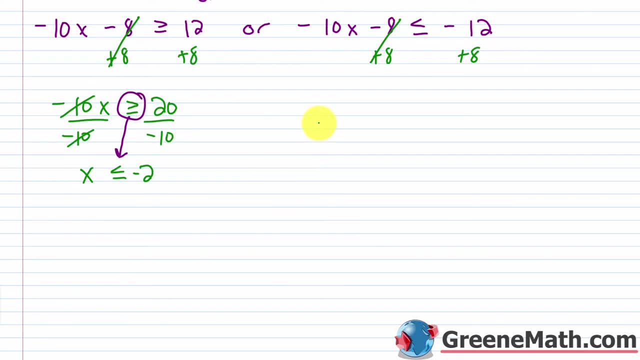 8 to each side to begin. that'll cancel. i'll have negative. 10x is less than or equal to negative. 12 plus 8 is negative 4.. let's go ahead and divide both sides by negative 10.. and if i divide by a? 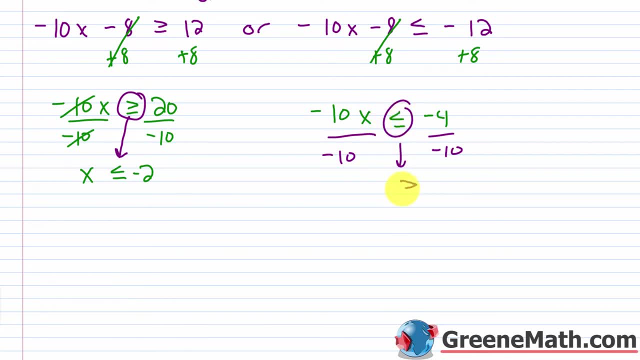 negative. i flip the direction of that inequality symbol, so it's going to be a greater than or equal to. now this cancels. x is greater than or equal to negative 4 over negative 10.. i know that negatives cancel, so this would be positive. each is divisible by 2. 4 divided by 2 is 2, 10 divided by 2 is 5.. so 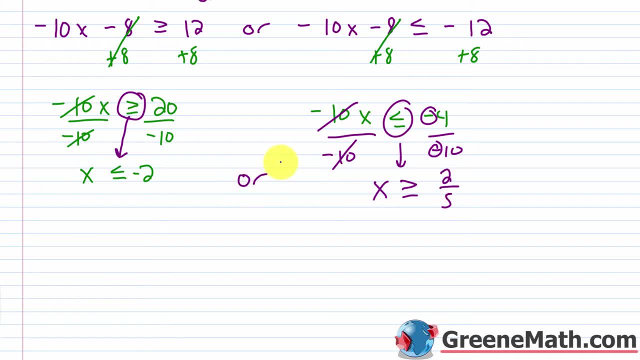 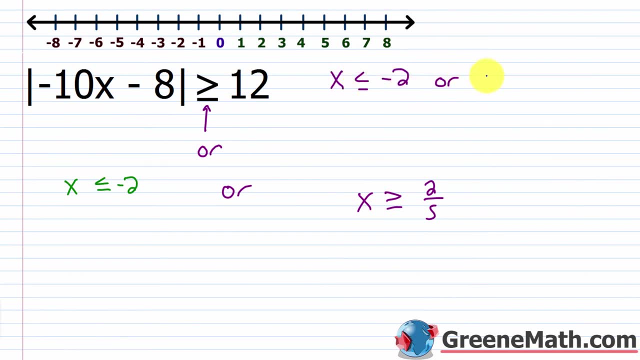 x is greater than or equal to 2- 5 there. so this is an or, and let's erase everything and notate this properly. so we have: x is less than or equal to negative 2, or x is greater than or equal to 2, 5.. 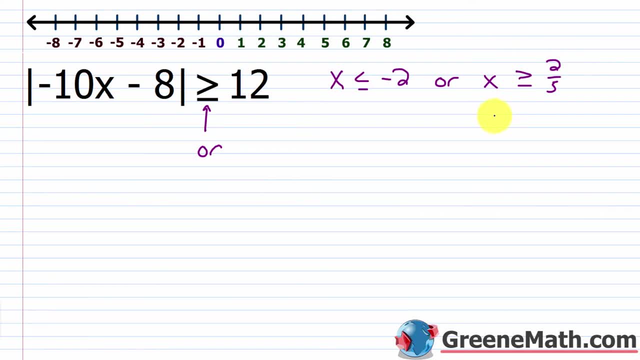 in interval notation. again it's the union of the two solution sets, so it's anything. we have negative, negative infinity out here as the smallest up to and including negative 2, so I'm going to use a bracket- and then the union with this guy, so including 2 fifths and anything. 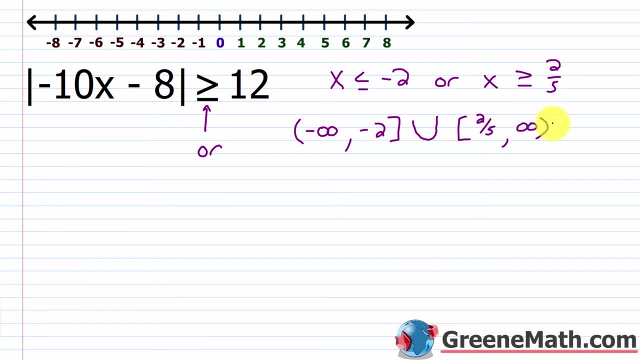 larger. So graphically I can find negative 2 on the number line that's here, put a bracket facing to the left and shade everything going this way. Okay now, 2 fifths doesn't have a notch, but 2 fifths is .4 as a decimal, so it's a. 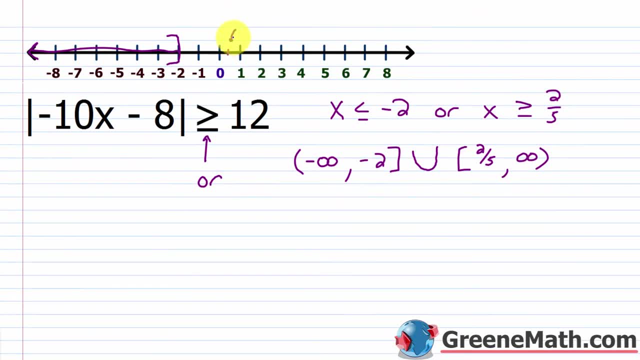 little bit less than a half. so let's just say it's like right there. let's say this is 2 fifths, and again it's anything that includes 2 fifths, so that value or larger. And again, if you have this on a test, your teacher's going to allow you to make notches. 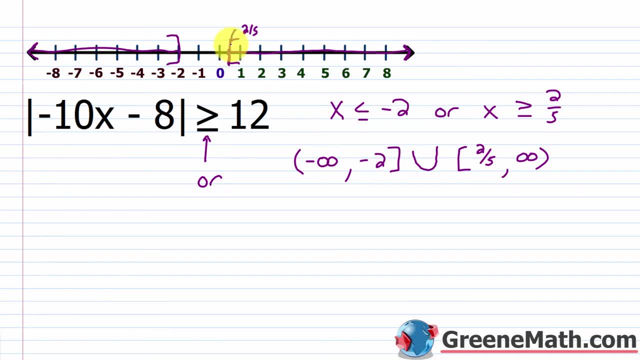 where they're on right. they understand that. So it's not perfectly at 2 fifths, but you know, you've notated where it is. That's the best you're going to be able to do. So, again, anything that is less than or equal to negative 2, along with anything that is. 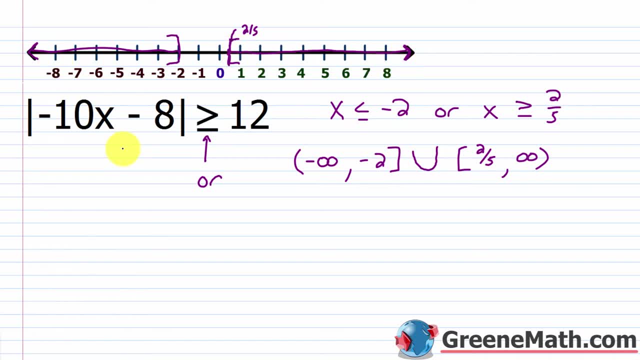 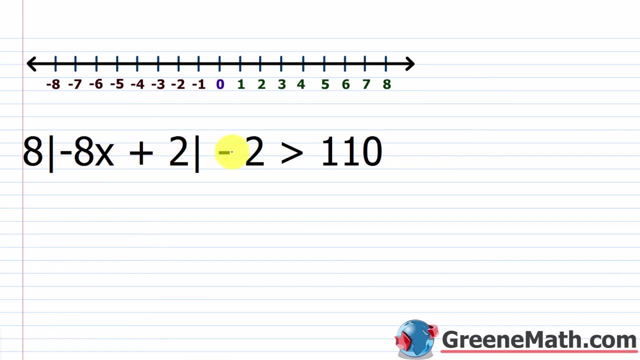 2 fifths or greater would be a solution for this inequality. All right, let's take a look at another one. So we have 8 times the absolute value of negative. 8x plus 2, minus 2, is greater than. 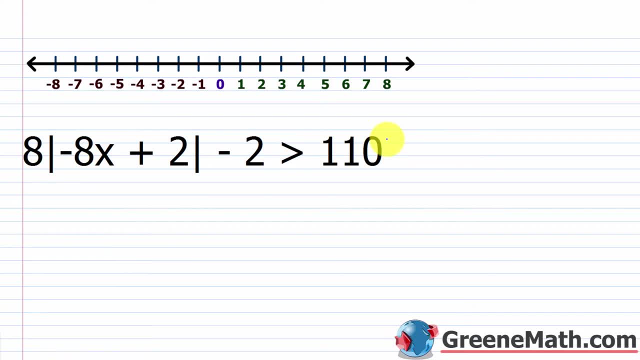 110.. So common mistake is, after you've seen these easy problems, you go through and you start saying, okay, well, 8 times, remove the bars. Negative 8x plus 2, minus 2 is greater than 110, or then you take this and you say, well, 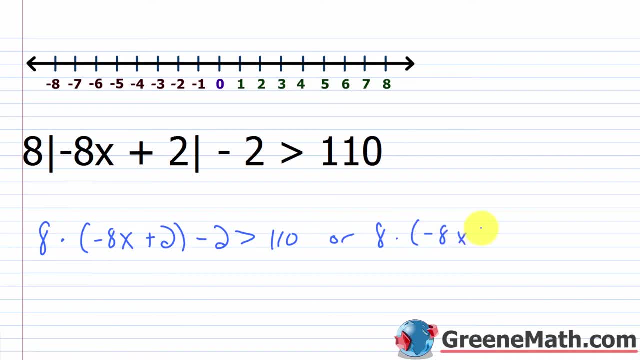 8 times and then, inside of parentheses, negative 8x plus 2, minus 2 is less than negative 110.. No, okay, Do not do this Wrong. You have to isolate the absolute value operation first. You want it to look like this: 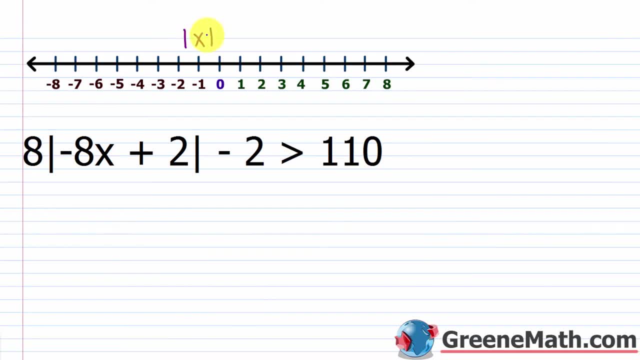 The absolute value of something. let's just say x, doesn't matter what it is- Is greater than some value k. So this x could be anything. It could be the absolute value of ax plus b, if you want to make it more complicated. 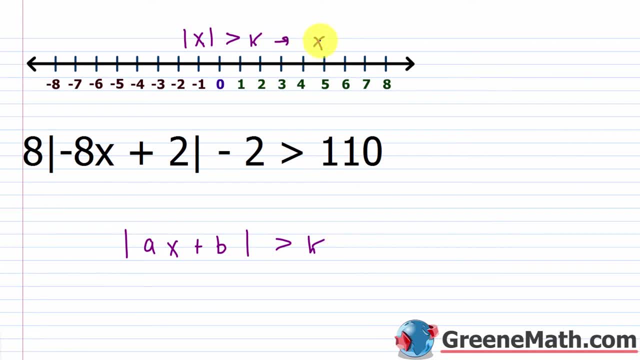 is greater than k. This leads to what x is greater than k or x is less than negative k. This, the more complicated example, just leads to: ax plus b is greater than k, or ax plus b is less than negative k. 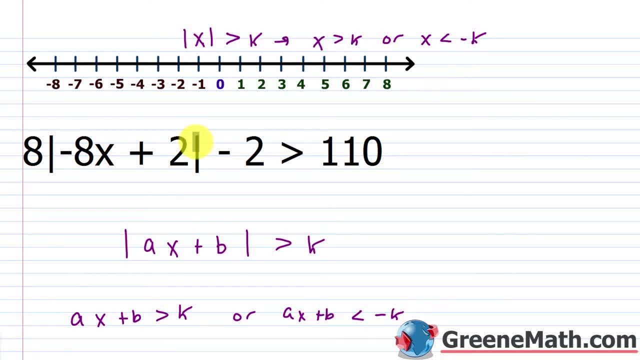 Okay, So the main thing here is to isolate The absolute value operation first and then just follow this formula here, Write it on a flashcard and keep using it. All right, let me erase this real fast and let's go ahead and simplify. 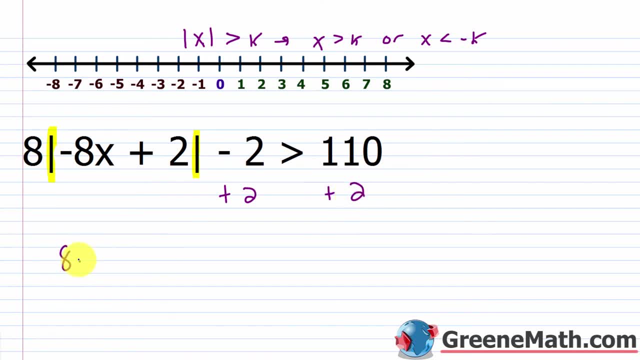 So I'm going to add 2 to each side. I'll have 8 times the absolute value of negative 8x plus 2.. This is greater. than 110 plus 2 is 112.. Now I want this by itself. 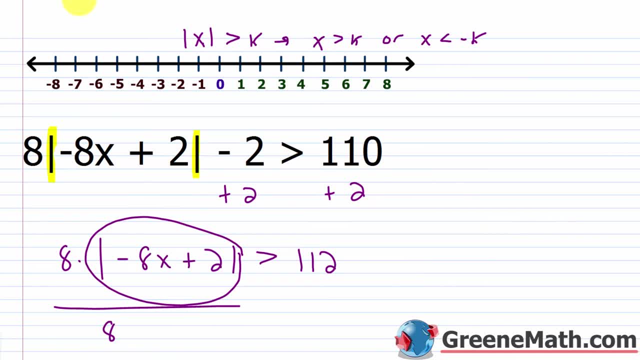 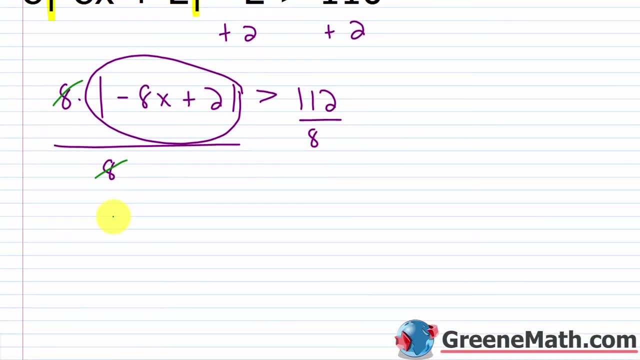 I have multiplication here, so I'm going to use division to get it by itself. Divide both sides, Divide both sides by 8, and so this will cancel. with this, I'm going to scroll down and get some room going and I'll be left with the absolute. 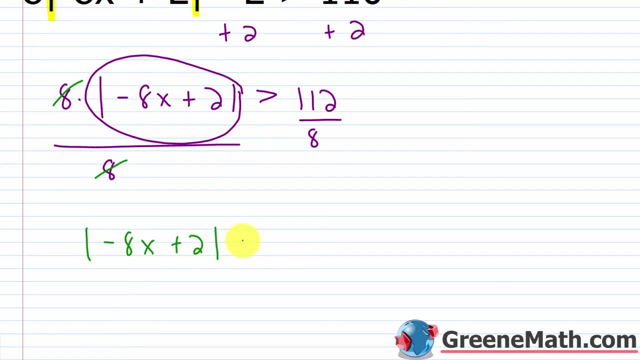 value of negative 8x plus 2 is greater than what's 112 divided by 8? Well, most of us don't know that off the top of our heads, but punch it up on a calculator and you'll get 14.. 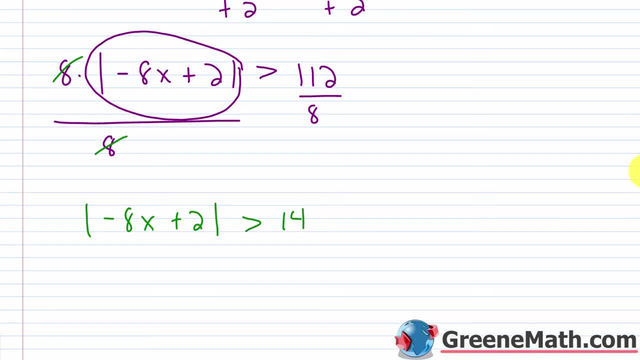 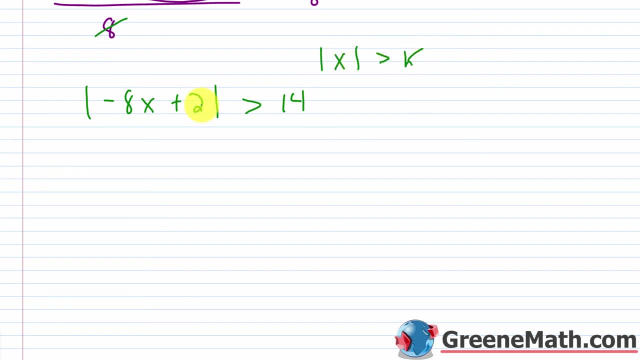 Now I have something that is matching again what I saw earlier. The absolute value of something, let's just say x, is greater than k. So the absolute value of negative 8x plus 2 is greater than 14.. 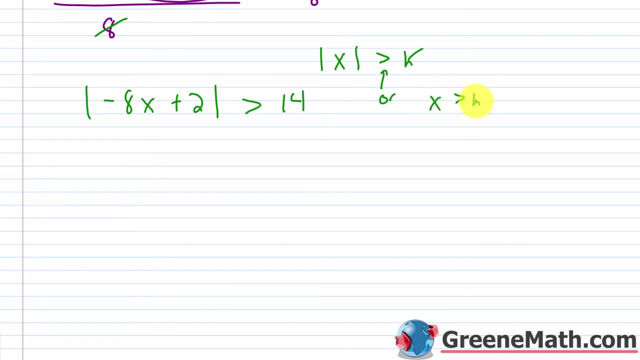 Remember. this sets up as: or So x is greater than k or x is less than negative k Same thing. This is or So we have negative. 8x plus 2 is greater than 14.. All I did was just remove the absolute value bars. 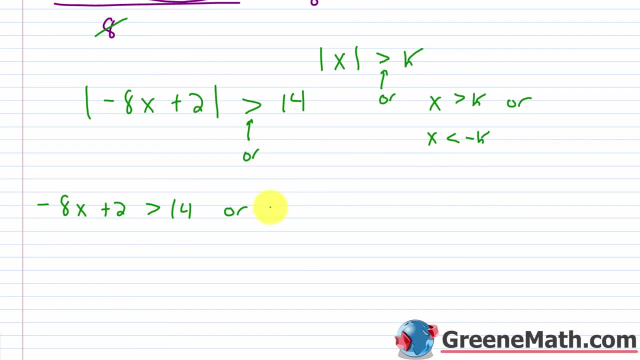 Then, or Remove the absolute value bars, so negative 8x plus 2. Flip this direction here. So this is a less. This is a less than Make this negative Negative 14. So you're basically good to go at this point. 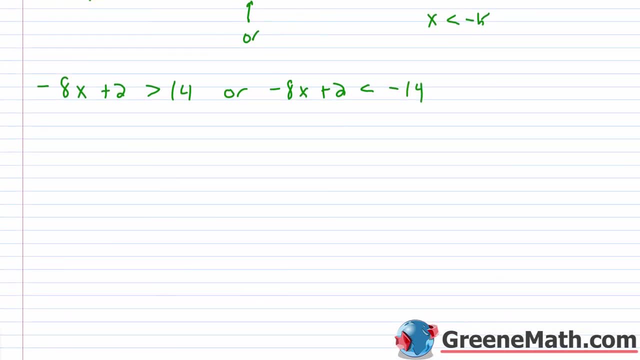 You just need to find your solution for this. So we're going to subtract 2 away from each side and that'll cancel. I'll have negative. 8x is greater than 12.. Divide both sides by negative 8.. You're going to flip the direction of this guy. 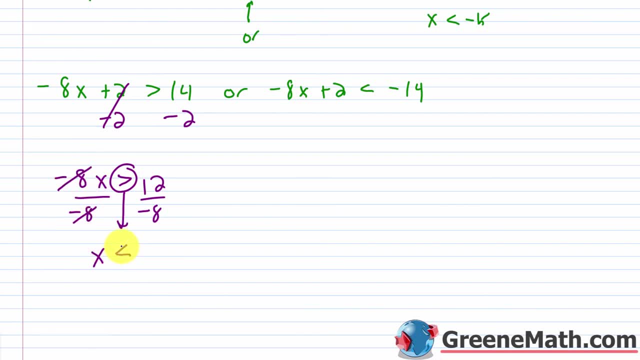 This will be a less than This cancels. with this I'll have. x is less than 12 over negative 8.. Each is divisible by 2.. In fact, each is divisible by 4.. So if I divide this by 4, I get 3.. 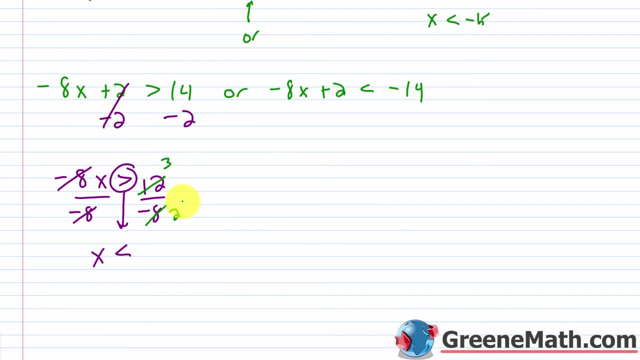 If I divide this by 4, I get negative 2. So let's put negative 3 halves And then let's look at the other guy. So if I subtract 2 away from each side over here, this is going to cancel. 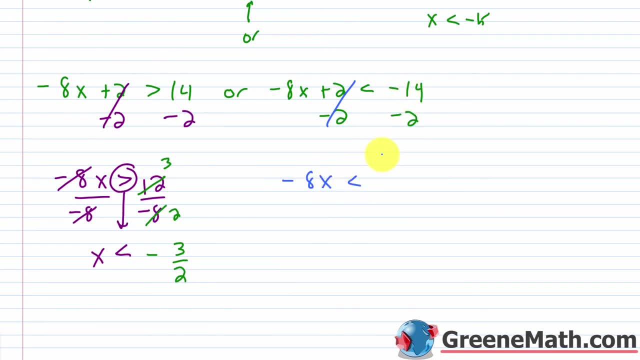 I will have negative. 8x is less than Negative. 14 minus 2 is negative 16.. Divide both sides by negative 8. So this will cancel with this And what I'll have is x, And I've got to flip this. 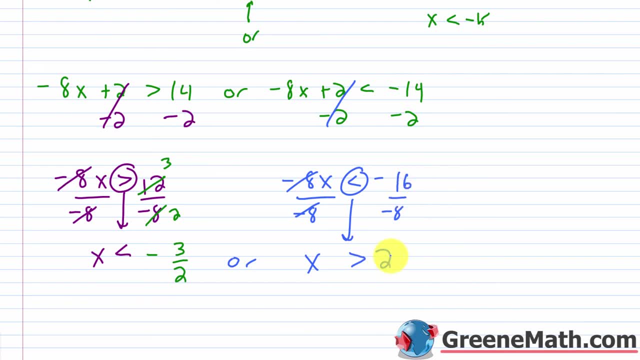 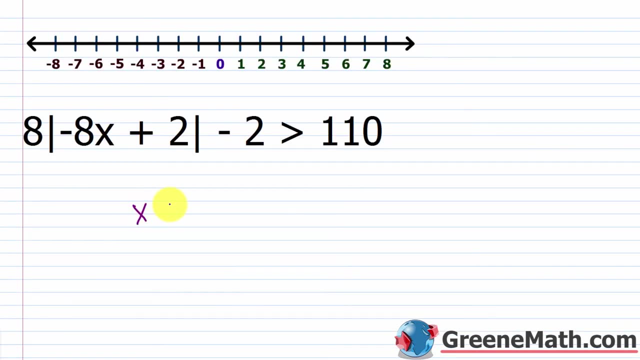 Is greater than Negative, 16 over negative, 8 is 2.. So x is less than negative 3 halves or x is greater than 2.. So again we found that x was less than negative 3 halves or x was greater than 2.. 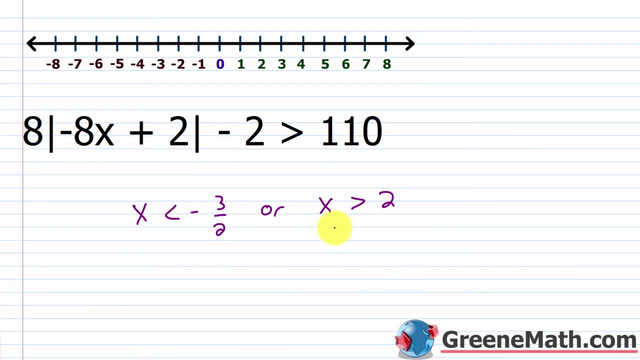 So in interval notation it's the union of the two solution sets, So coming from negative infinity up to, but not including negative 3 halves, And the union with this other guy After 2, right, Anything larger, out to infinity. 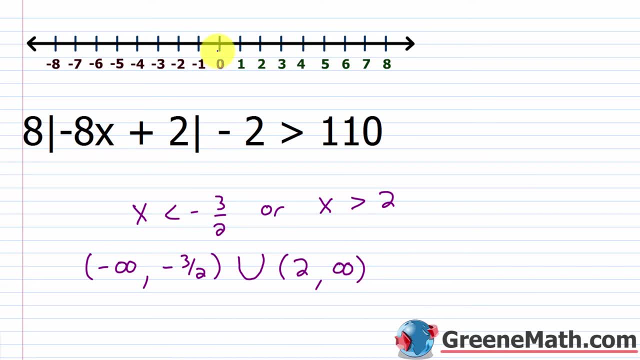 Graphically I don't have a negative 3 halves, But negative 3 halves is negative 1.5.. So it's between negative 1 and negative 2.. So let's just say it's right there. This is negative 3 halves. 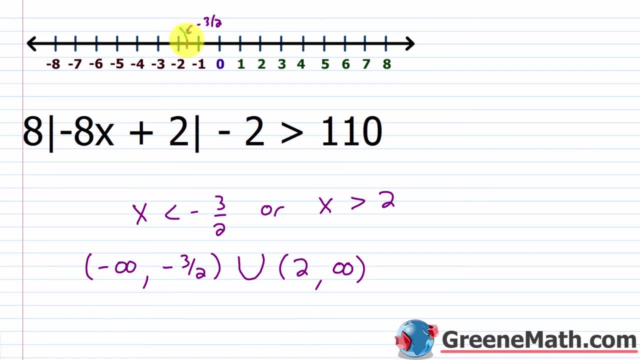 It would be anything less than that. So I'll put a parenthesis facing left, Shade everything to the left And then anything larger than 2.. So put a parenthesis at 2. And we'll shade everything to the right. 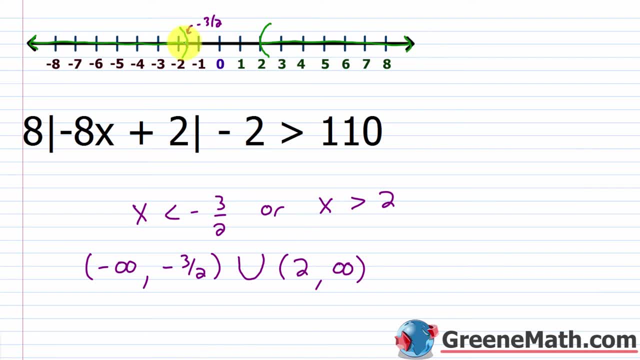 So again, x can take on any value that is less than negative 3 halves, Or it can also take on any value that is larger than 2.. Alright, let's take a look at one now where we have a less than. 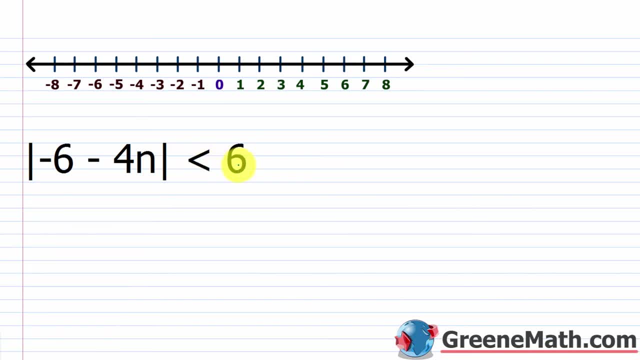 So we have the absolute value of negative: 6 minus 4n is less than 6.. So again, if we see something in this format, The absolute value of x is less than k. It's a compound inequality with and. 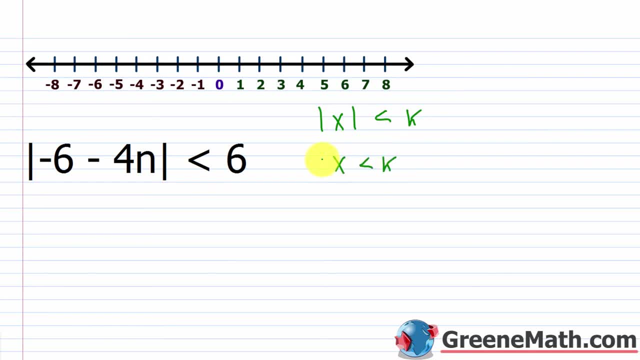 So x is less than k, But it's also greater than the negative of k. Okay, so you have: x is less than k and x is greater than the negative of k. So I'm going to take this part right here. 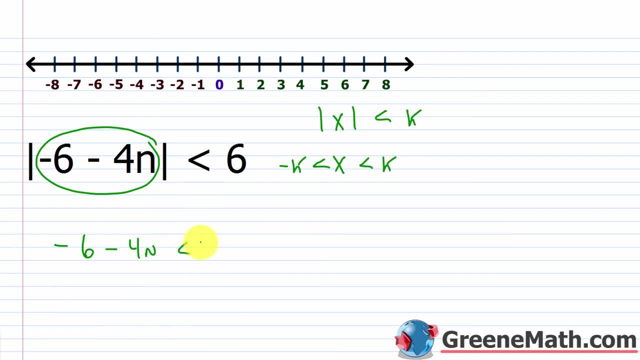 And I'm going to say negative- 6 minus 4n is less than 6.. So the same as it looks right here. Just drop the absolute value bars Then, and Okay, now you have, and because you have a less than, 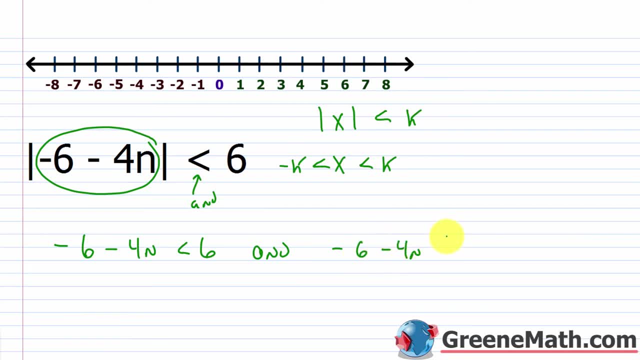 It's also true that negative 6 minus 4n is greater than Flip the sign just like you do before, Make this negative. So negative 6.. So negative 6.. So negative 6 minus 4n is greater than negative 6.. 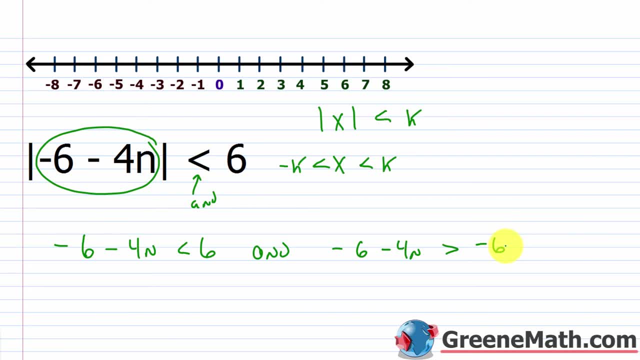 So we can write this as a three-part inequality. Make it easy on ourselves. So we have negative 6 minus 4n in the middle. It's greater than negative 6. And it's less than positive 6. So I can just erase this. 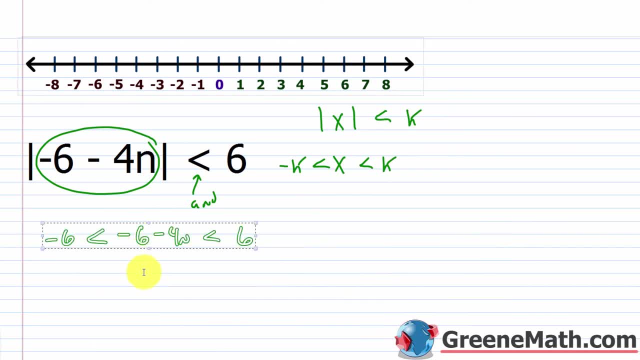 And I can drag this up here And again. if you're wondering where this came from, I've showed it multiple times. But it's basically that we take the negative of this, So negative of negative 6 minus 4n. 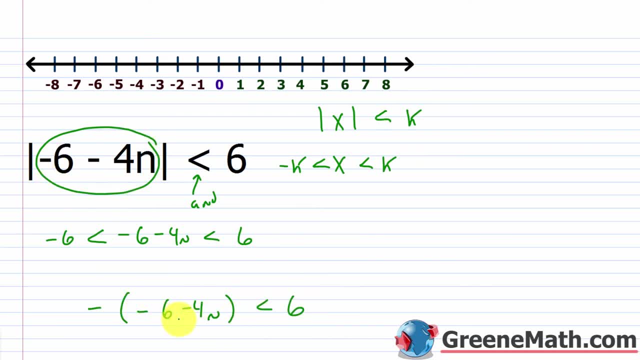 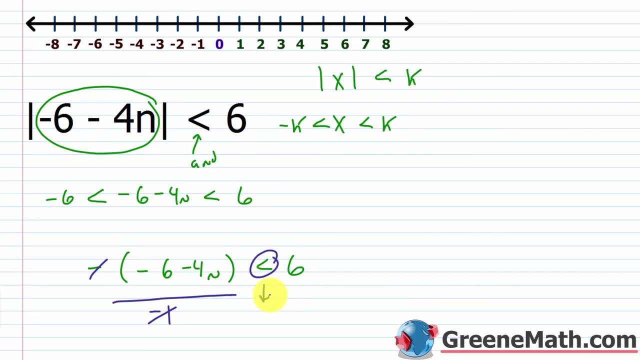 This is less than 6. Because of the absolute value operation, that would work as well. And then we divide both sides by negative 1. So this cancels. That makes me flip the sign, And then this becomes negative 6.. 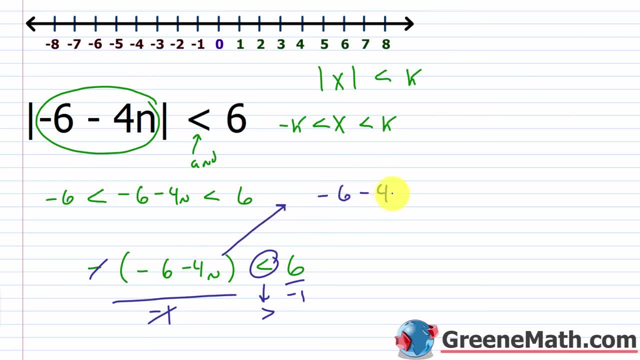 So we have this guy right here, Negative 6 minus 4n, The sign is flipped And then we have negative 6.. So that's where this part right here comes in. Let me erase all this now And let's just attack the problem. 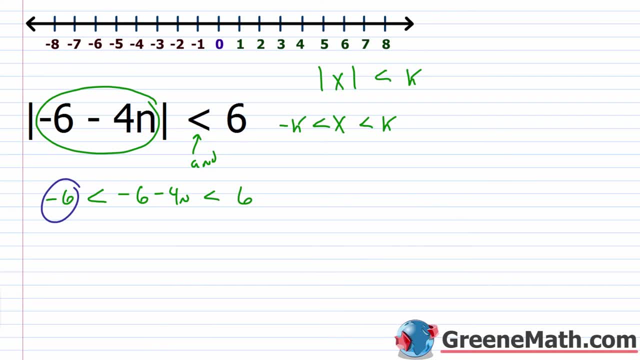 So if I Solve this three-part inequality, I do the same thing to each part. I'll add 6 over here and over here, So that'll cancel. Become 0.. That'll cancel. I'll have negative 4n. 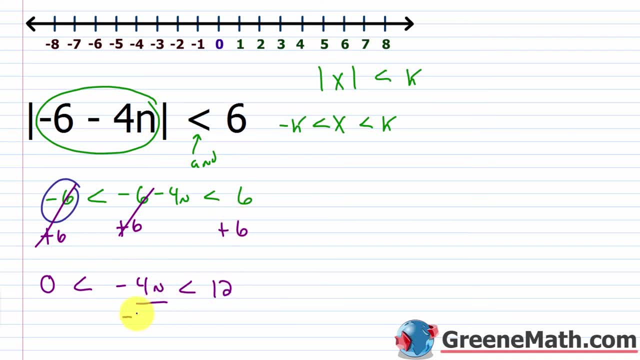 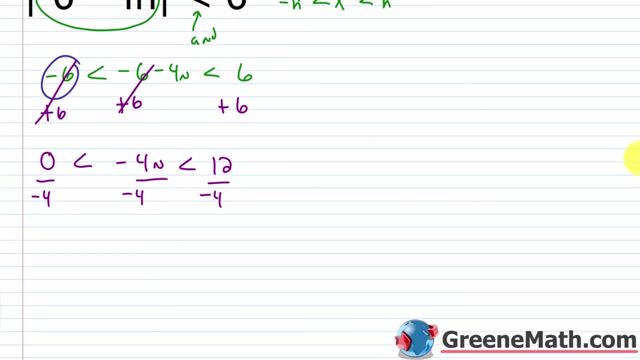 Is less than 6 plus 6 is 12.. So I divide each part by negative 4.. So I can isolate n And what's going to happen is, Again, I've got to still flip the direction When I have a three-part inequality. 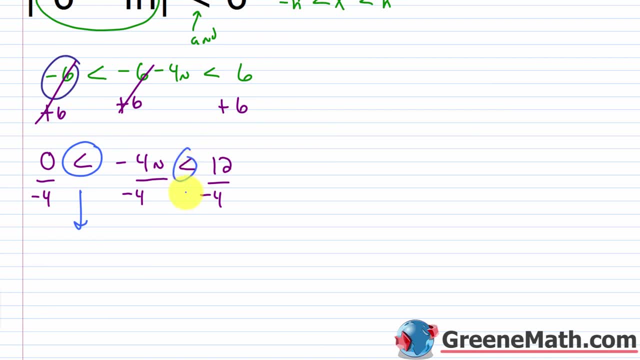 And I divide by a negative That doesn't change. So this gets flipped And this gets flipped. So this is greater, Then this is greater, Then this cancels with this And I'll have n, So n is less than. 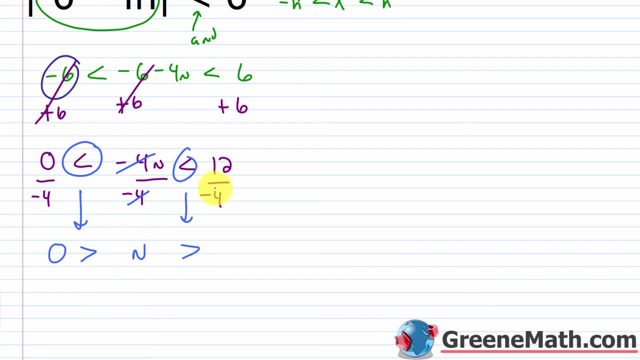 0 divided by negative 4 is 0. And it's greater than 12 divided by negative 4 is negative 3.. So generally we don't leave it in this manner. We rearrange it to where it's, in the direction of the number line. 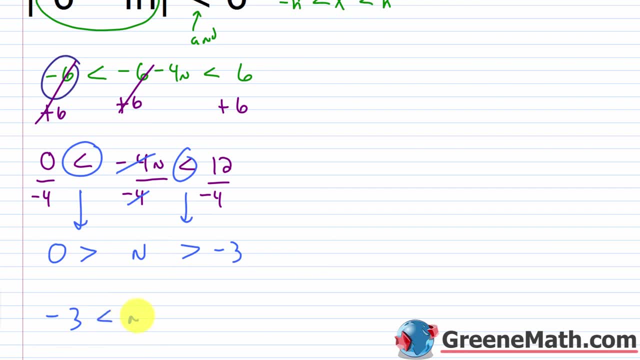 So negative 3 would be here. Of course, that's less than n, And we know that n is less than 0.. So let's take this solution up And we're going to graph it And use it To write. 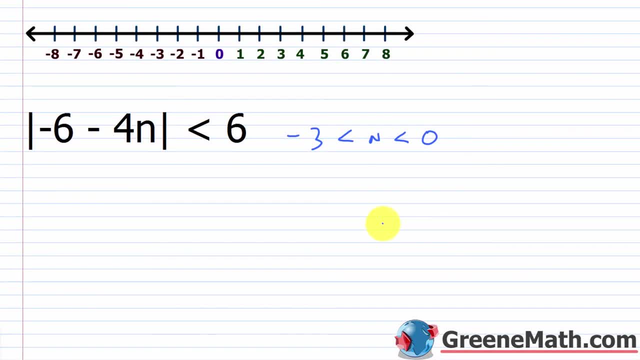 An interval, So n is greater than negative 3. And less than 0.. So here's negative 3.. So it's greater than that And it's less than 0.. So it's between negative 3 and 0.. 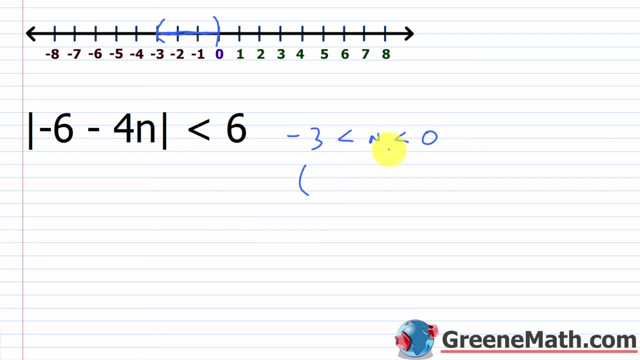 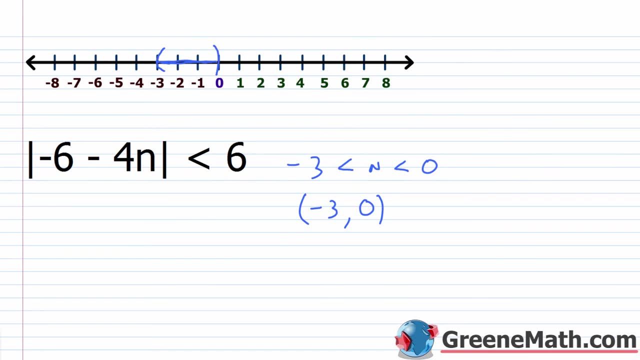 So that's what it looks like graphically And an interval notation. I just have the interval Greater than negative 3.. But less than 0. Just like that. So n again can take on any value that's greater than 3.. 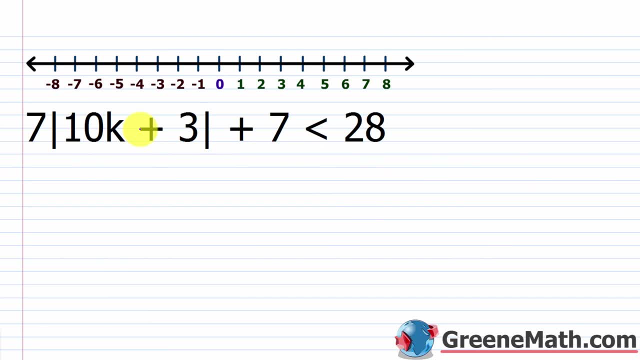 But less than 0.. Alright, for the next one. We're looking at 7 times the absolute value of 10k, Plus 3. Plus 7 is less than 28.. So again, I want to isolate the absolute value operation. 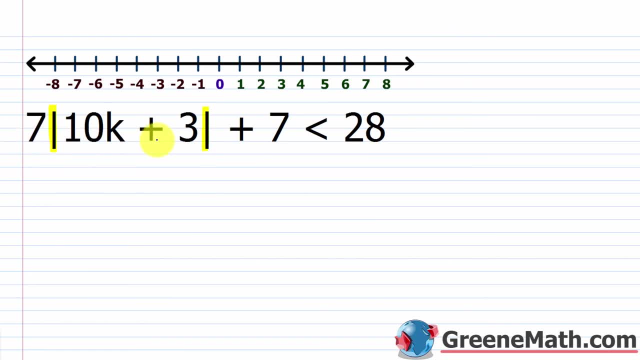 Before I do anything, Don't make the mistake of just trying to apply the rule Before you have isolated the absolute value operation. So I want to subtract 7 away from each side first. I'll have 7 times the absolute value of. 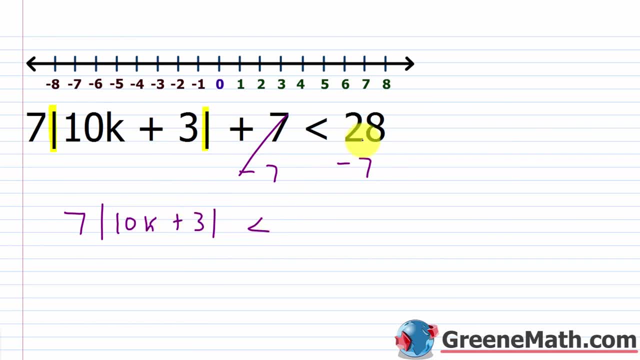 10k plus 3. This is less than 28 minus 7 is 21.. So now I can divide both sides by 7, and when I do that, this will cancel. with this I've isolated my absolute value operation. 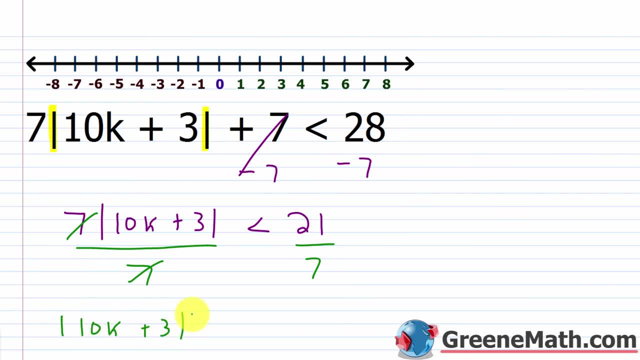 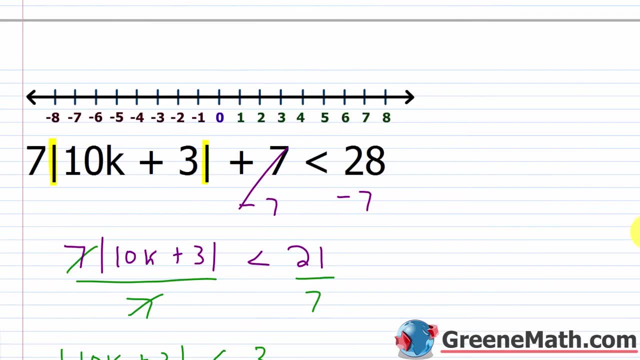 It's the absolute value of 10k plus 3.. And this is going to be less than 21 divided by 7 is 3.. So now I can go ahead and apply my little formula: Remove the absolute value bars, So I'll have 10k plus 3.. 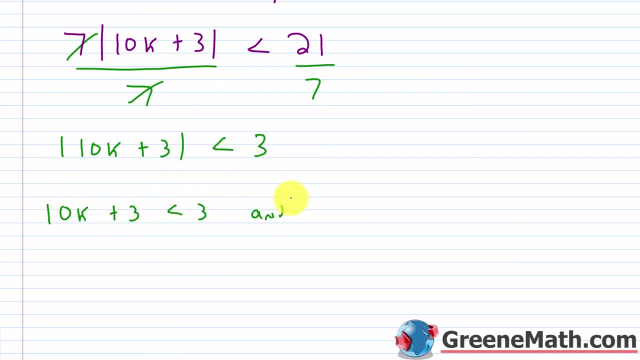 And then it's just less than 3.. And the other scenario would be that 10k plus 3, remove the absolute value bars, flip the direction of the inequality symbol so it's greater than, and then make 3 negative. 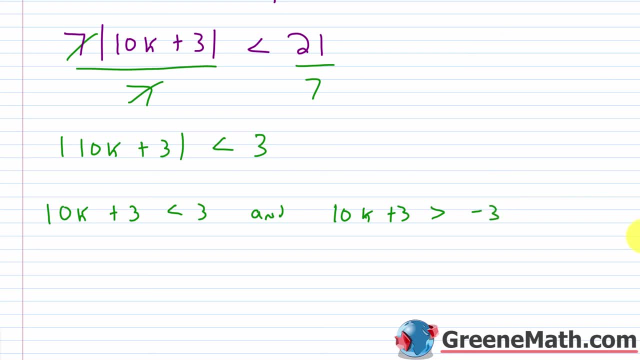 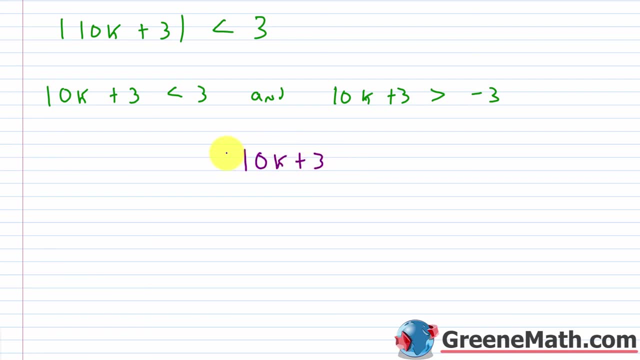 So negative 3.. And again, to make this easier on yourself, write it as a 3-part inequality. So go ahead and write this as 10k plus 3 is greater than negative 3 and less than 3.. So let's subtract 3 from each side. 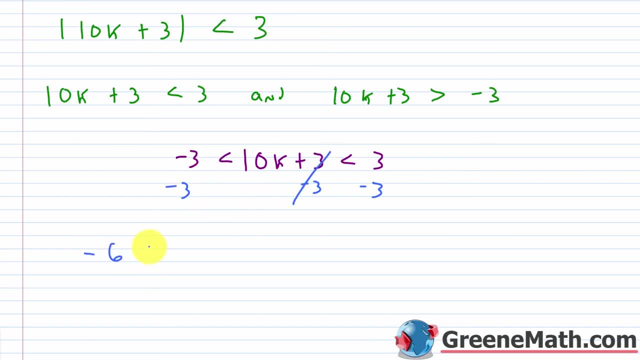 So this will cancel Negative. 3 minus 3 is negative 6. This is less than We'll just have 10k now And it's less than 3 minus 3 is 0.. Divide each side by 10.. 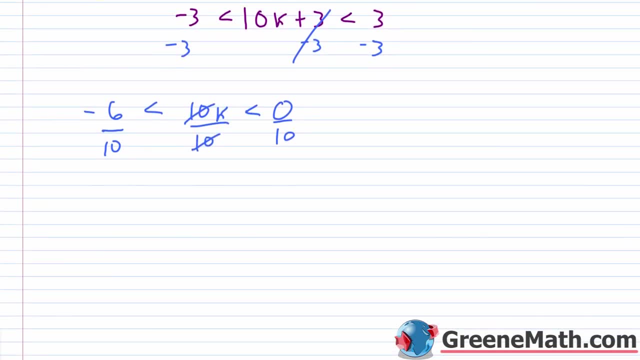 This will cancel with this And I'll have k in the middle by itself, which is what I want, And it's going to be greater than negative 6 over 10.. I know it's negative 6 is divisible by 2.. 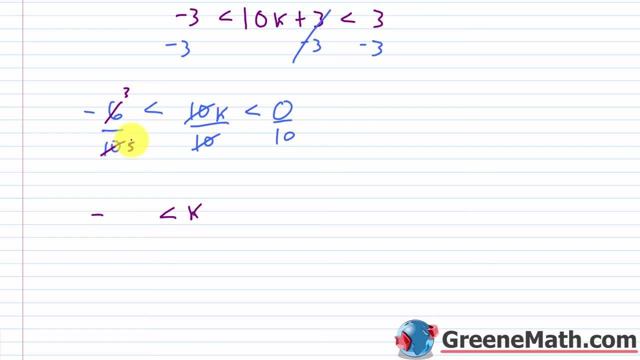 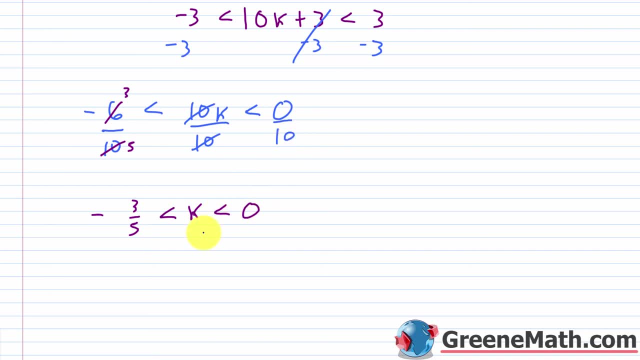 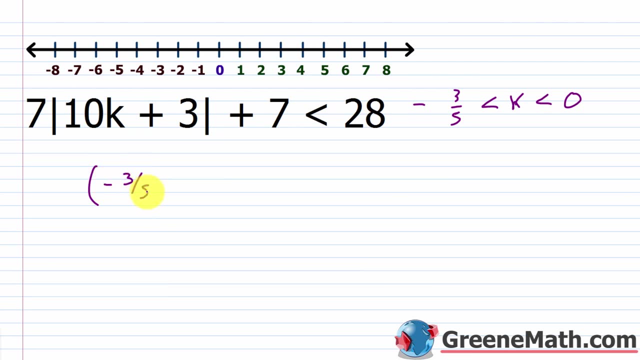 So then less than 0. So k is greater than negative 3 fifths and less than 0. So in interval notation that's not including negative 3 fifths up to, but not including 0. So it looks like that. 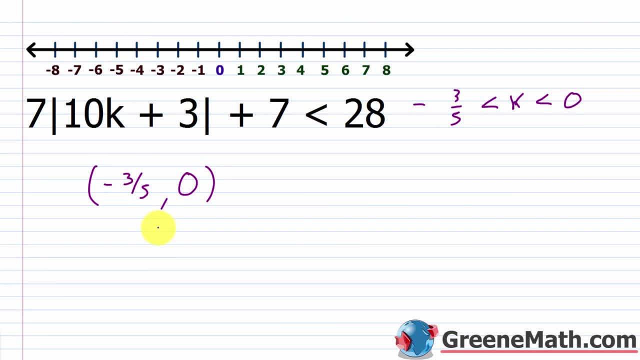 And then on a number line, where is negative 3 fifths? Well, it's negative 0.6.. So if you look between 0 and negative 1, it'd be a little bit past negative 0.5.. So let's say about right there. 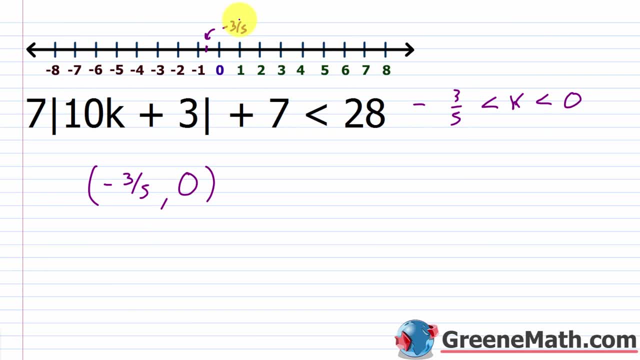 We could say this is negative 3 fifths, So here's 0.. So what I would do is I would put a parenthesis here facing to the right, one here facing to the left. It's kind of a small area on our number line. 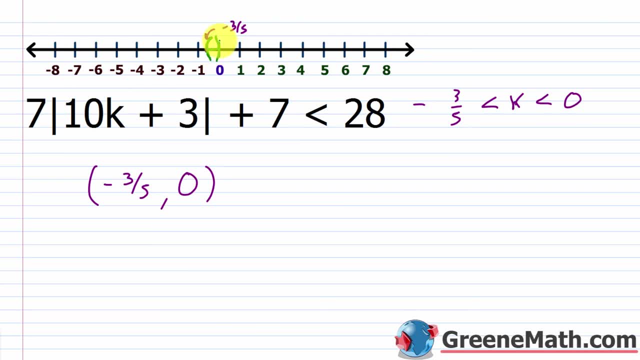 We'd shade everything in between. So again, k can be anything that is greater than negative 3 fifths, up to and not including 0. So anything in that range between, again, negative 3 fifths and 0.. 4.5. 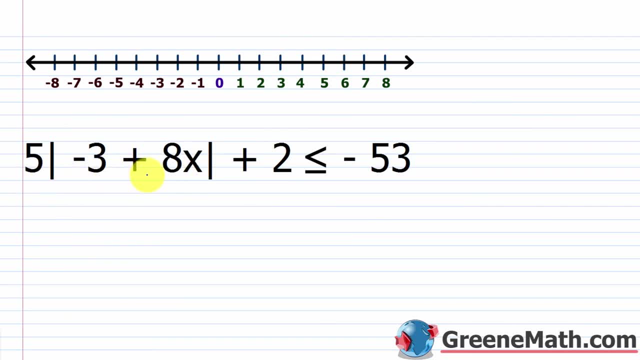 And then we're going to look at: we have 5 times the absolute value of negative 3 plus 8x plus 2 is less than or equal to negative 53. So again, I want to isolate the absolute value operation first.